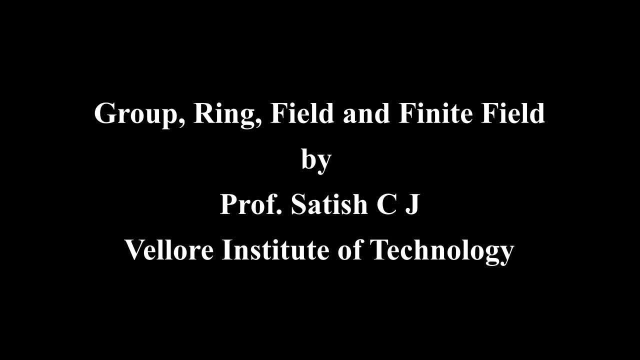 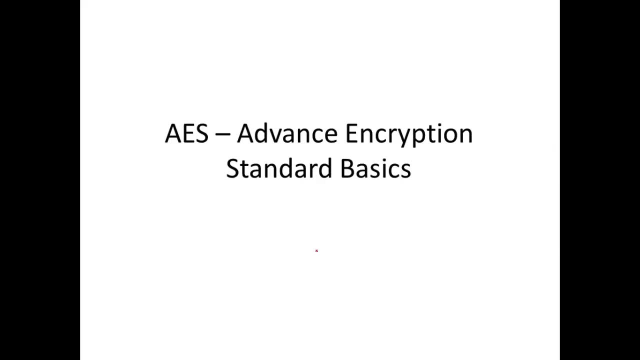 In our previous session, we were looking at DES data encryption standard. We looked at some variations of DES that is double DES and triple DES. We have understood the weakness of DES and we looked at why DES is insecure. And we are now going to look at the next advanced encryption standard that has superseded DES and that is called AES. AES is nothing but advanced encryption standard and this is the latest standard that is ruling the world right now. And almost any kind of encryption that is happening is happening using AES. But to understand AES, we need to understand certain basic mathematical concepts and this session we are going to try and understand all these basic mathematical concepts that will help us to understand advanced encryption standard in depth. So, these are the concepts that we are going to learn and these concepts fall under abstract algebra. Some of you might have learnt all these concepts in your schools, but let us again refresh these concepts. We will start with understanding what is a group, then we will go to what is a ring, what is a field and we will understand finite fields. Finite fields are very important because when you talk about advanced encryption standard, advanced encryption standard is based on finite fields. So, to understand finite fields, we need to understand group, rings and fields. 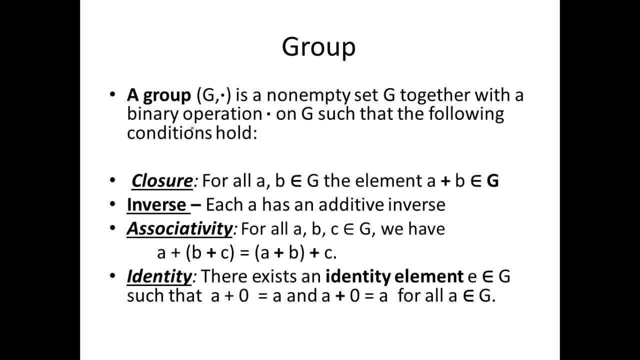 First we will start with group. So, what is the group? A group is very simple, it is nothing 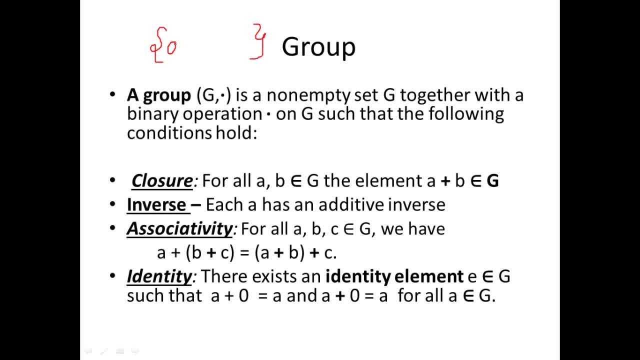 but a set of elements. Let us consider A B C to be the set of elements. The set of elements can be anything. 1. Set of elements 2. Set of matrixes 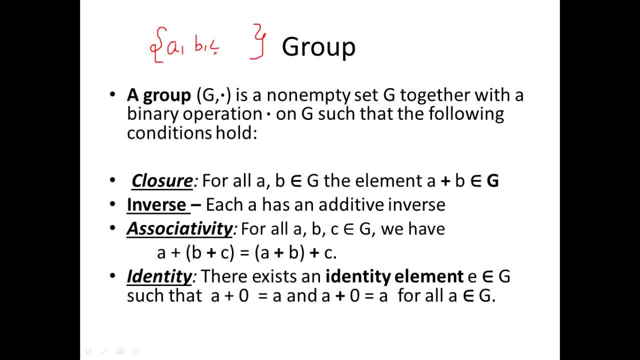 it can be a set of polynomials a set of rational numbers set of real numbers set of integers anything so it's just a set of elements and on this set of elements we are just going to apply 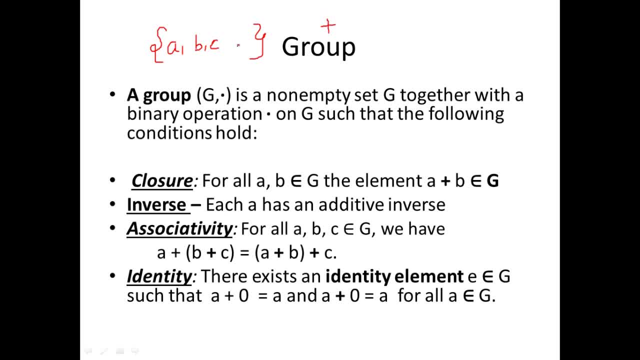 an operation let's consider addition if i take addition and apply it on any two elements and i should be able to achieve or satisfy all these properties by applying that operation on the set of elements then i will say that is a group so let me repeat this it's nothing but a set of 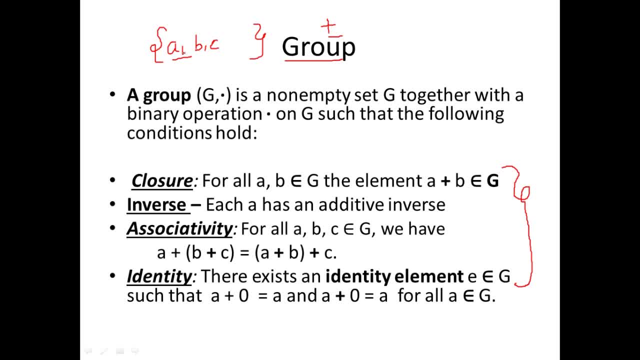 elements and an operation we take this operation and when we apply that on the set of elements we need to satisfy all these axioms so when all these properties are satisfied you call those set of elements as a group so let us take an example let us take the set of all integers set of all integers is set of all integers is 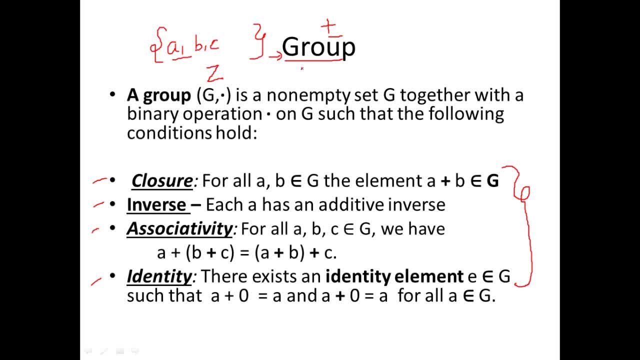 set of all integers is denoted with the set and let's take set of all integers so we can have a set like this minus three minus two minus one so it's an infinite set right so it's zero one two sets it's a set of all integers i'm just giving some numbers here and we'll take this operation addition and we'll try and see whether these axioms satisfy this set for any a b belonging to this set the element a plus b should also belong to this set so if you take any two integers and add the result five is also part of this set so this is true for a set of integers each has an additive inverse so what is this additive inverse say two plus minus two is equal to zero so every element you take has an additive inverse so this is also true for a set of integers associativity that is a plus b plus c is equal to a plus b plus c this is also true right two plus three plus five the result is going to be equal to two plus three plus five no matter how you do addition is associative so this also holds true for the operation on the set of integers identity what is that for every element you take that element you add a zero then you're going to get the same element this is true three plus zero is equal to three and zero plus three is equal to three so there is an identity element that is also part 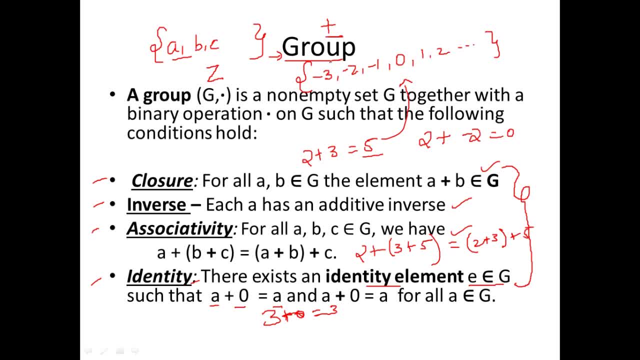 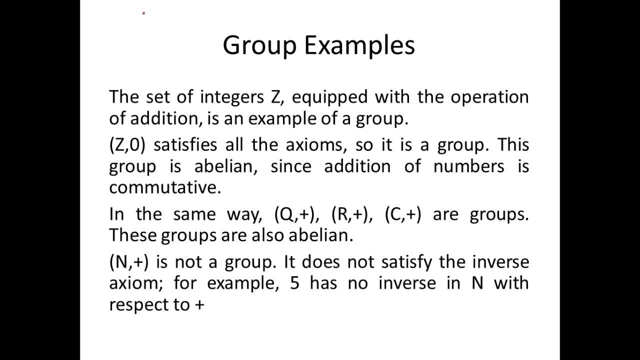 of this set so any two elements you take and you apply an operation the result also should be part of that set that is the most important criteria here and when these properties are satisfied we can call this set of integers to be falling under group so likewise you can take the set of rational numbers and the addition operation it's going to satisfy all these properties you can take the set of complex numbers and the addition operation it's going to satisfy all these properties set of real numbers and all these operations is going to satisfy so all these sets which satisfy these four axioms with respect to the operation addition we can call them to be a group there's one more thing in abstract algebra we don't have a subtraction say we can take two numbers say five minus three they say there is no subtraction it is nothing but five plus minus three so they consider this to be an additive inverse so there is nothing called subtraction here everything even this kind of an expression is treated as five plus minus three so that's why in our previous slide for the group i was only talking about this operation addition though it is also applicable for subtraction so here are some of the examples for groups i told you set of integers a cube with the operation of addition is an example for a group we have seen that 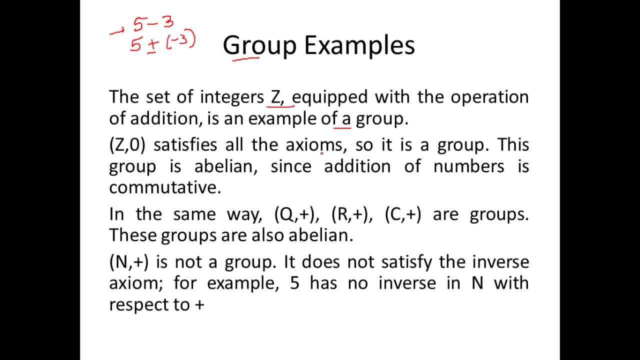 and here is one more thing z comma zero satisfies all the axioms that is 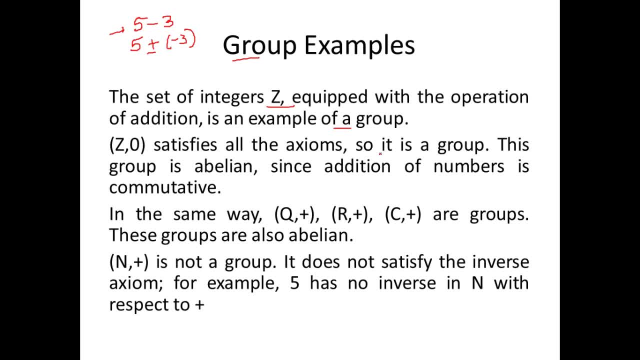 teachers along with zero satisfy all the axioms so it is a group we have seen that this group is an abelian group since addition of numbers is commutative so a plus b is equal to b plus a so this axiom is satisfied so you're going to say the group with all these axioms satisfied to be 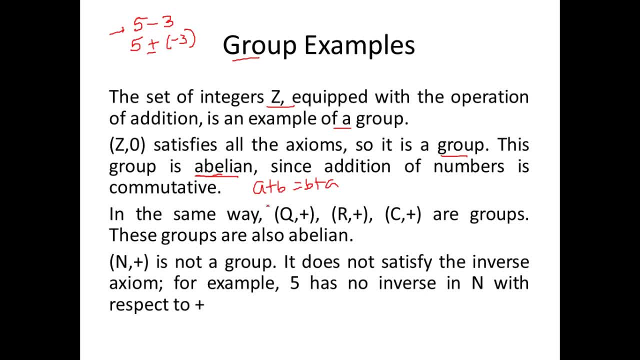 abelian group so in the same way q represents here represents your set of rational numbers and r represents set of all real numbers c represents set of all complex numbers so when you take set of all these numbers and you apply 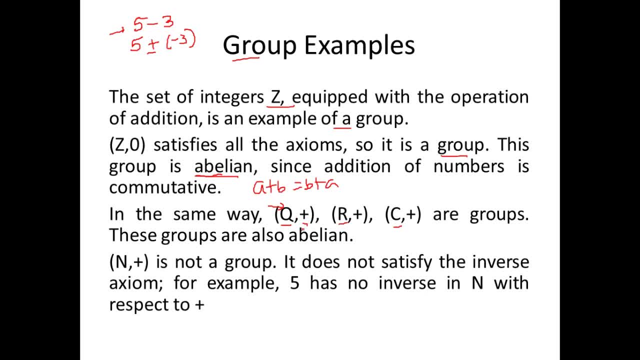 this addition operation you're going to have all these axioms satisfied so we say all these sets come under the concept of groups in abstract algebra let's take an example for instance 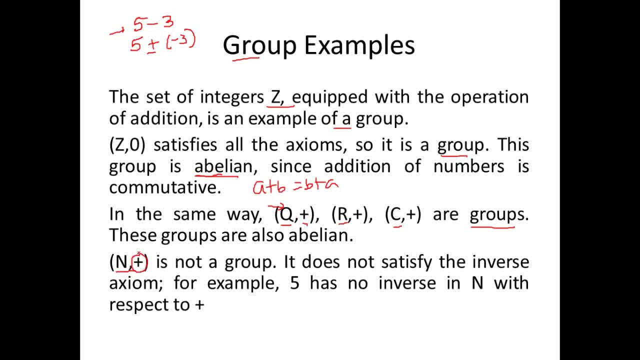 set of all natural numbers with the operation addition does not come under a group so let's take set of all natural numbers it starts from one two three 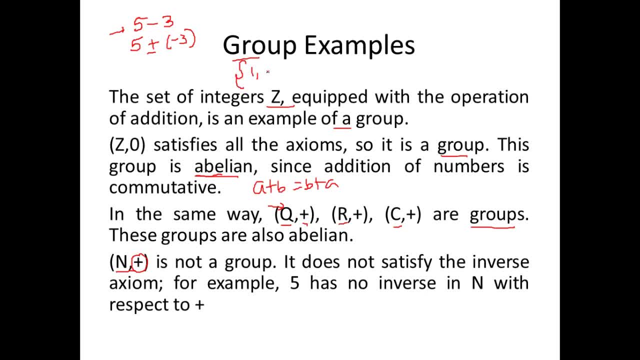 and it goes right it doesn't come under a group because these numbers don't have an additive inverse say you you you can't go and find two plus minus two that is equal to zero right 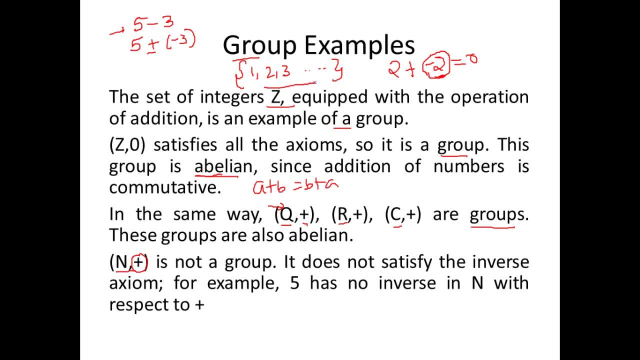 here you don't have minus two minus two is not part of the set of natural numbers so since the elements here they don't have an additive inverse we can say that all the natural numbers with this 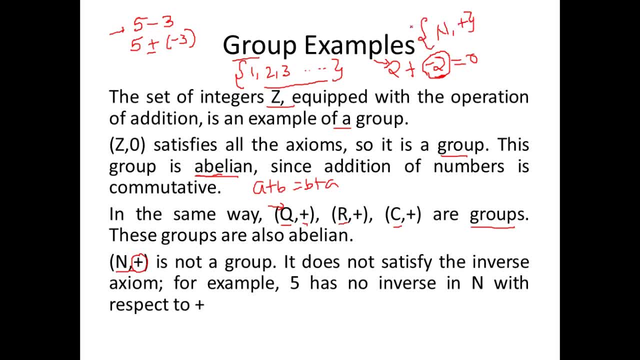 operation plus does not form a group okay 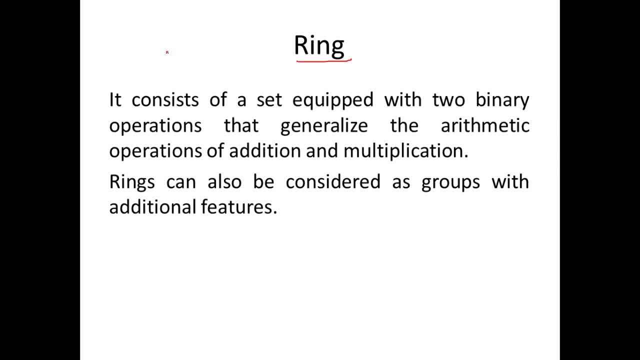 what is a ring a ring is nothing but again it's a set of elements and these set of elements can be anything as told earlier in our earlier group example we are looking at only one operation plus here 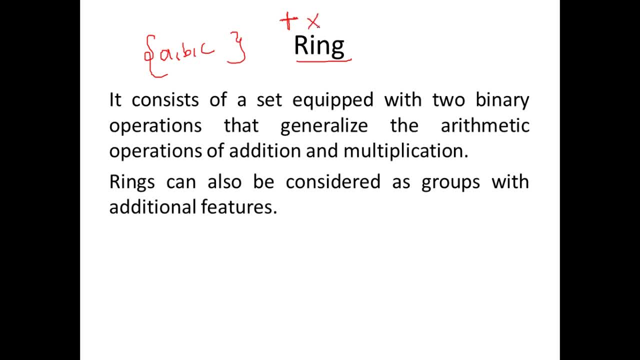 these elements are also going to support another operation that is multiplication so when a set of elements are going to support these two operations and the result is also part of the set then we can always consider that to be a ring so what is a ring it consists of a set equipped with two binary operations that generalize the arithmetic operations of addition and multiplication rings can also be considered as groups with additional features 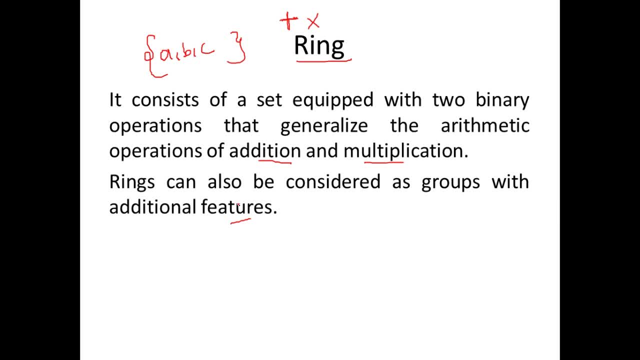 for groups we just support the addition operation whereas in rings the multiplication operation is also supported so it means when you take two elements and you multiply the third element is also part of the set so multiplication property is also supported in rings 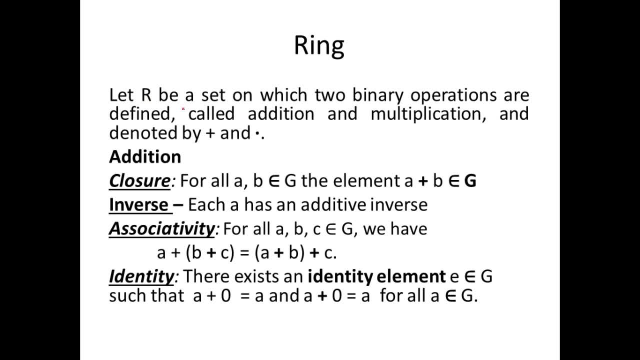 let's take a look at the definition for rings a ring are a set on which two binary operations are defined that is addition and multiplication and it is denoted by plus and a dot and with respect to addition operation these axioms should 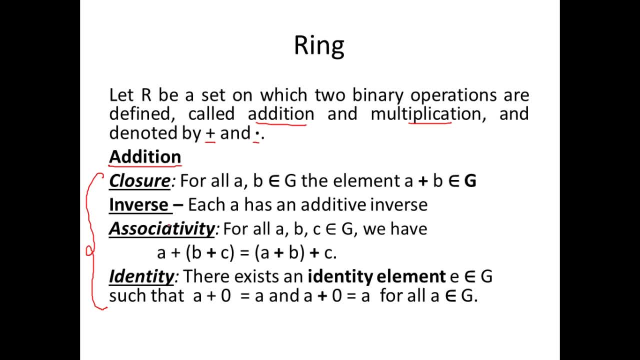 be satisfied these axioms are again from the group so closure so you take again let's take set of all integers it contains both negative and positive numbers right so set of all integers you take any two numbers and you can divide them, you can have negative and negative, and the result includes both positive and negative numbers. the result also belongs to the set so that is closure after all, 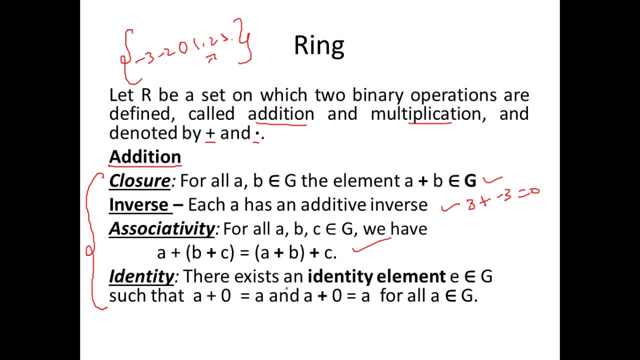 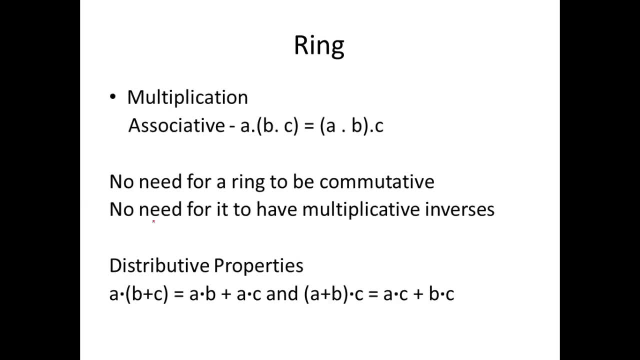 first true for theит does not add up to zero, then it is added with any element in the set returns the element and with respect to multiplication, the element should satisfy the associativity rule that is a dot b dot is equal to a dot b dot is equal to zero . red part does not add up to any element i mean which one enter we will ask you so understand the feelings if it is non deductible if weullンタ Notre. 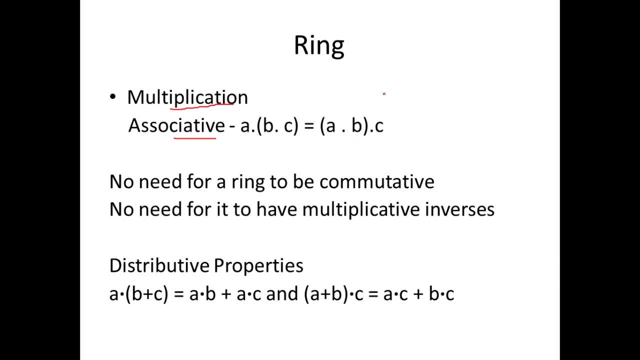 equal to a dot b into c. So, when this additional property is also satisfied by the elements then we can say the elements the set of elements form a ring in abstract algebra and there are certain 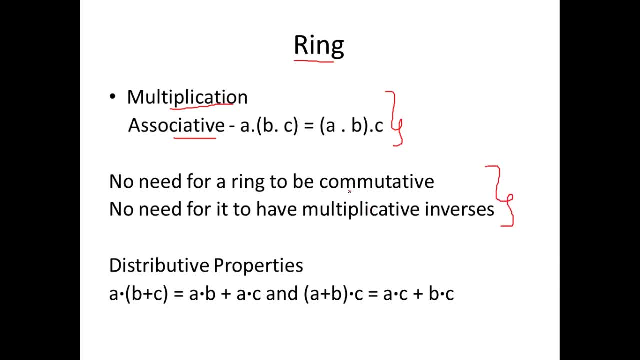 things here no need for a ring to be commutative with respect to multiplication. We do not expect a dot b to be equal to b dot a this is not a requirement for a ring and no need for it to have multiplicative inverses. So, these are two properties that are that that is not mandatory for a ring and both multiplication and addition together should satisfy the distributive property. 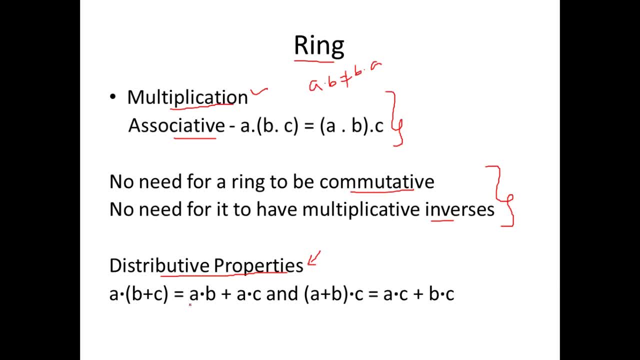 So, for a ring this should be satisfied a dot b plus c is equal to a dot b plus a dot c and a plus b dot c is equal to a dot c plus b dot c. So, the distributive property wherein multiplication and addition together combined should be satisfied for a for the elements in the ring. 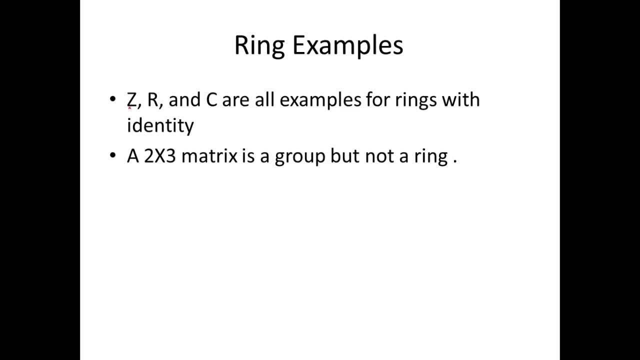 So, let us take some examples for rings set of all integers yeah they are satisfying all the properties axioms with respect to multiplication and addition. So, with respect to addition they satisfy closure identity inverse associative even when you take two elements say 3.2 is equal to 2.3 commutativity with respect to multiplication is also satisfied. So, z also forms a ring likewise it applies for real numbers and complex numbers too. So, these are examples for rings with identity. So, here is one good example wherein 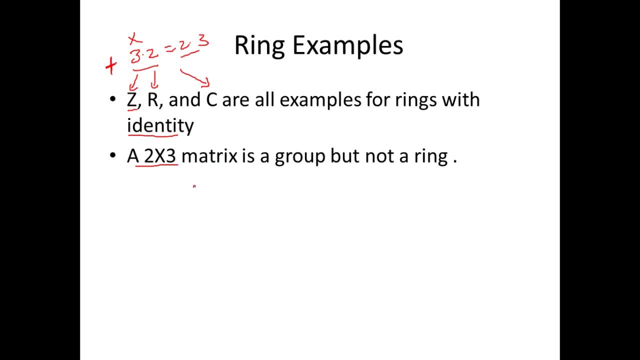 a set is a group but it is not a ring. Let us consider a set of elements wherein each element is a matrix. So, it has two rows and three columns something like this. 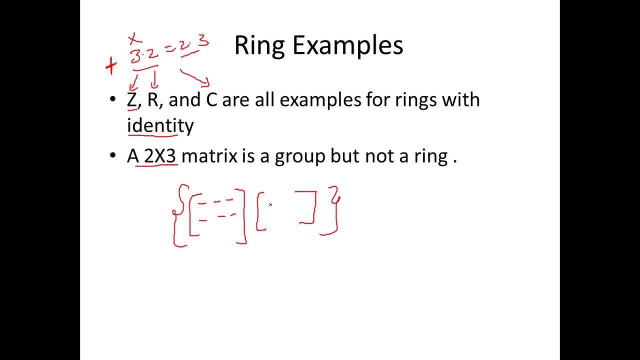 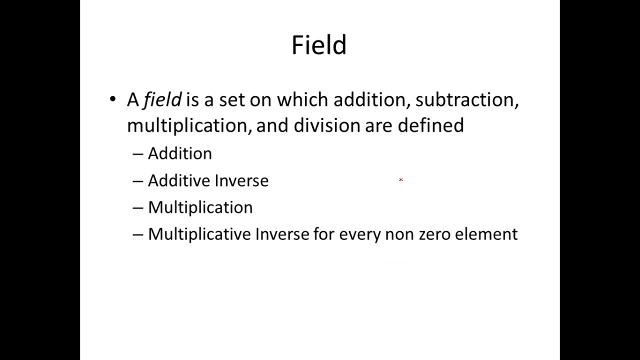 So, all the elements are matrices here and these matrices do not form a ring. Why so? Because when you multiply a two cross three matrix you cannot multiply a two cross three matrix with the two cross three matrix right. You cannot do that to multiply a two cross three matrix we need a three by two matrix. So, only we can multiply a two cross three matrix with that two cross three matrix. So, let me tell you if you have one two three and four five six your two cross three matrix you cannot multiply that with again another two cross three matrix. You need a matrix like this, i.e. whereas, you have 8 9 10 and 11 12 13 3 by 4 your 2 cross 13 matrix with your two cos 3 matrix. So, only then you can take every element and then you can multiply and add it right. So, multiplication is not supported in the set of 2 cross 3 matrices, but addition is fine when you add 2 2 cross 3 matrices you are going to get a 2 by 2 cross 3 matrix. So, that is fine, but whereas when you talk about multiplication, multiplication is not supported. So, the set of all elements that form a 2 cross 3 matrix is a group, but it is not a ring. So, we have finished what is a group, what is a ring. 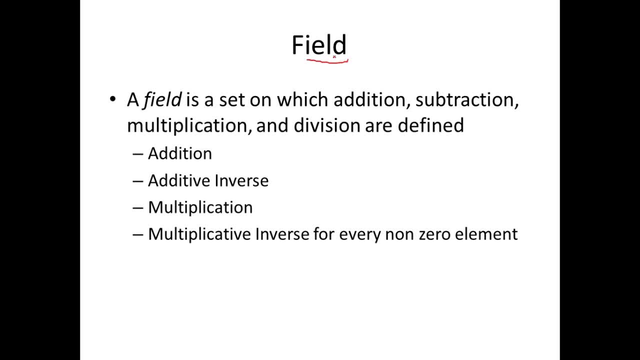 Now, let us take a look at what is a field. A field is again an extension of a ring. Say on a group what all you apply addition and subtraction and what you applied on a ring, on a ring you applied addition, subtraction and subtraction. Multiplication. So, when the set of elements satisfy all these operations it becomes a ring whereas when you talk about a field it is like an extension of a ring too. What is the only operation that is remaining? So, a field is nothing, but it supports a set of elements that support addition, subtraction, multiplication and division. So, if you have a set of elements, what is a field is nothing, but again a set of elements. 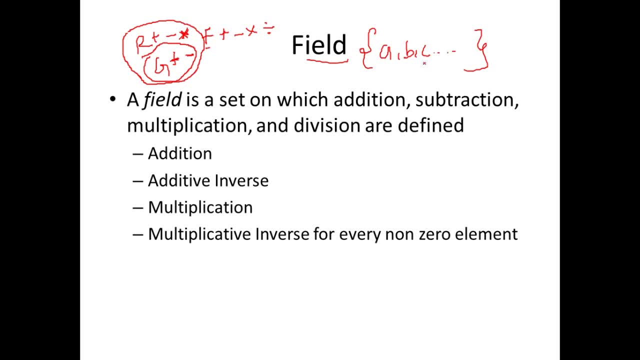 And what all operations are being supported? That is addition, subtraction, multiplication, division. If only three operations are supported that is a ring. If only the first two operations are supported what is that? That is a group. So, now we are looking at a field wherein 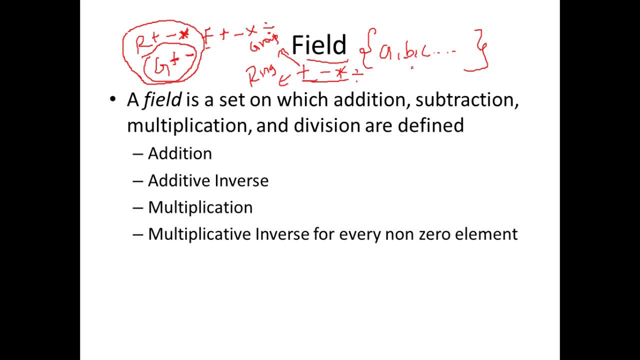 no matter even when you perform division the result should also be part of the set actually. 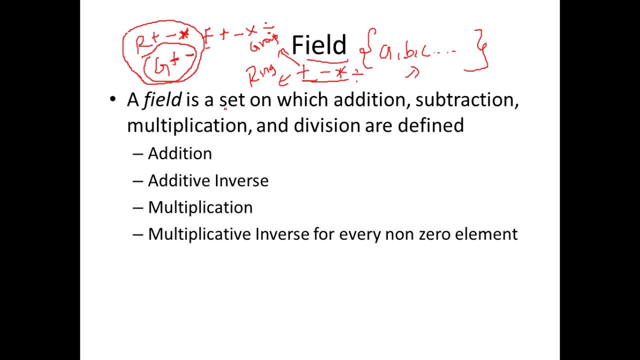 A field is a set on which addition, subtraction, multiplication and division are defined. But with abstract algebra as I have already told you there is addition, but there is no subtraction we call that additive inverse. Say when we say 5 minus 3 we actually say it is 5 plus 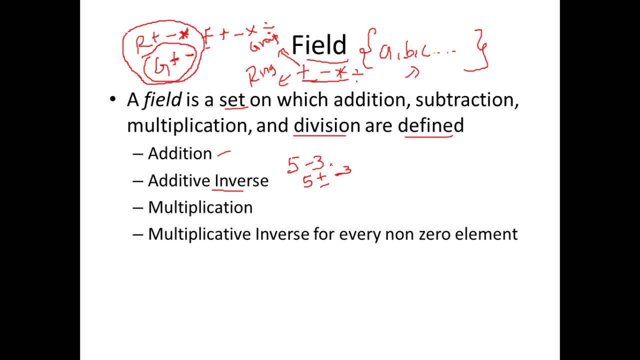 minus 3. So, even subtraction is looked like addition here. Multiplication we know what is multiplication. And we don't say division instead we say multiplicative inverse. Say 3 divided by 5 is nothing, but 3 into 1 by 5 wherein 1 by 5 is considered to be the multiplicative inverse. 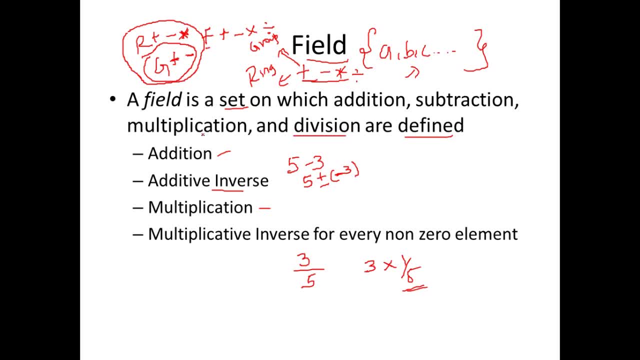 When we talk about field, a field should support all these operations that is addition, additive inverse, multiplication. multiplication and there should be a multiplicative inverse for every non-zero element 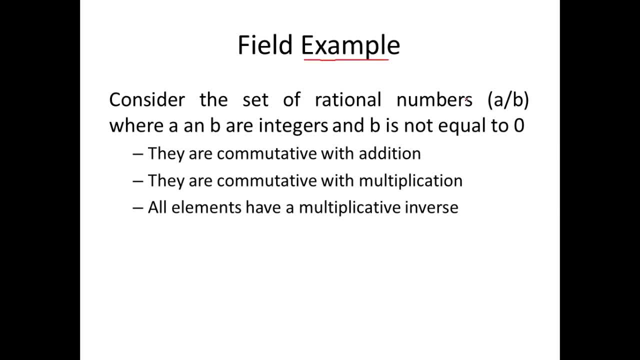 let's take an example for a field set of all rational numbers what are rational numbers it's nothing but two integers of the form a by b where b is not equal to zero so we all know what is a rational number and they are commutative with addition so a by b plus c by d is equal to 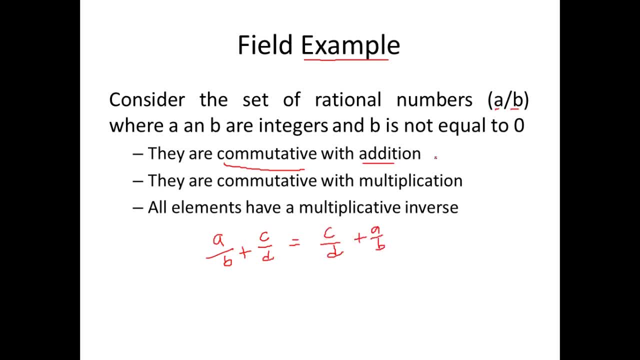 c by d plus a by b so rational numbers satisfy the first rule here commutative with multiplication you agree that say a by b star c by d is equal to c by d star a by b right so commutativity is also satisfied and rational numbers are commutative with respect 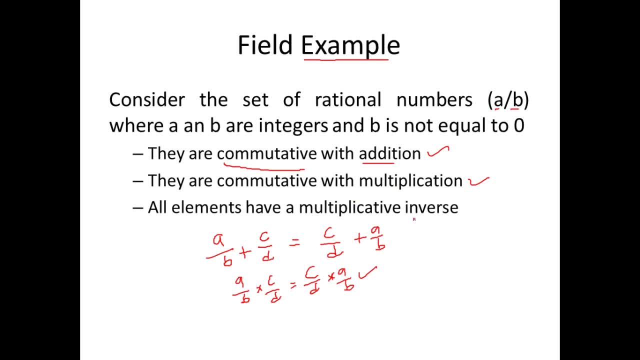 to multiplication all elements have a multiplicative inverse so what is that say 2 by 3 what is the multiplicative inverse of 2 by 3 it's 3 by 2 so the final result will be 1 product will be 1 and every element has a multiplicative inverse 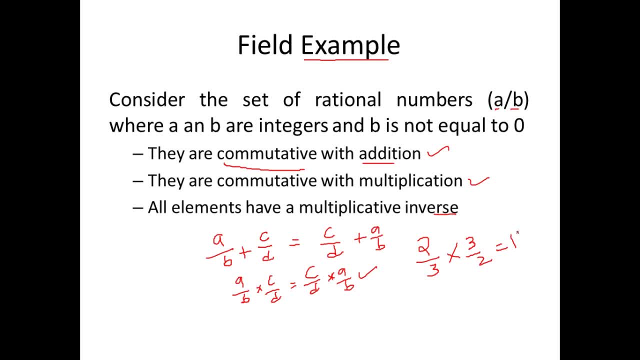 is the final result that is the meaning here and even this the result say this number which we say is the multiplicative inverse is also part of this set of rational numbers right if 2 by 3 is a rational number 3 by 2 is also a rational number so an inverse also is part of the set that is very important so when when you take set of all rational numbers all these three 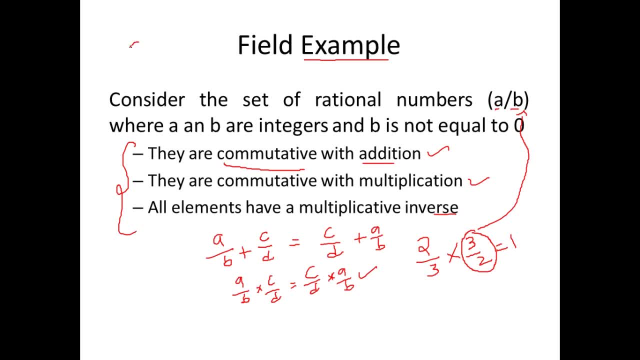 properties are satisfied set of all rational numbers that is denoted by q with respect to all these operations plus minus 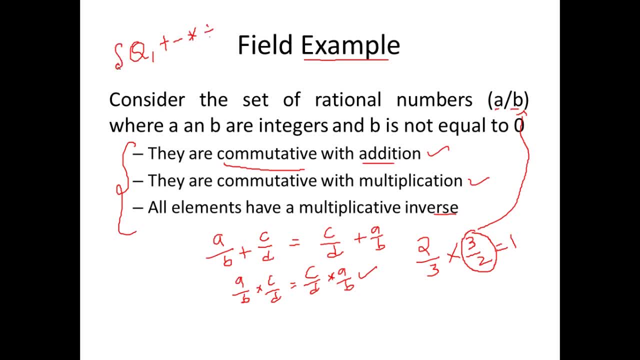 star division that becomes a example for a field. Let us take another two sets which do not form a field. For instance the set of all integers say you take an integer 5 what is the inverse of 5 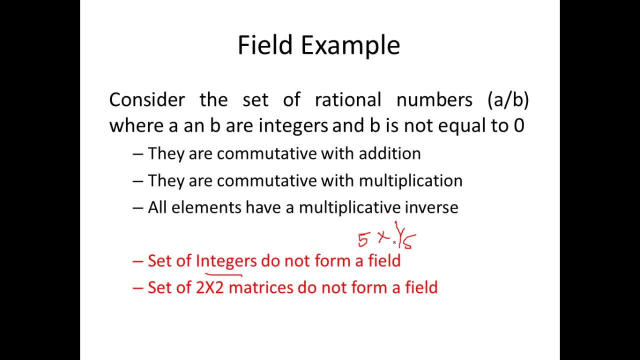 it is 1 by 5 and 1 by 5 is not an integer right. So, this inverse is not part of the set so it 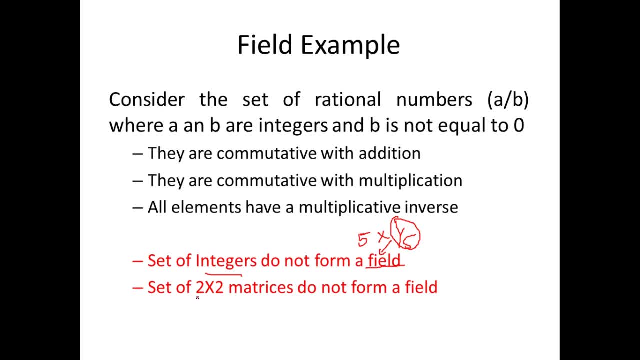 does not form a field. Likewise 2 cross 2 matrices do not form a field because they are not commutative. So, you multiply matrix A by B is not always equal to B into A. So, that is why 2 cross 2 matrices do not form a field. 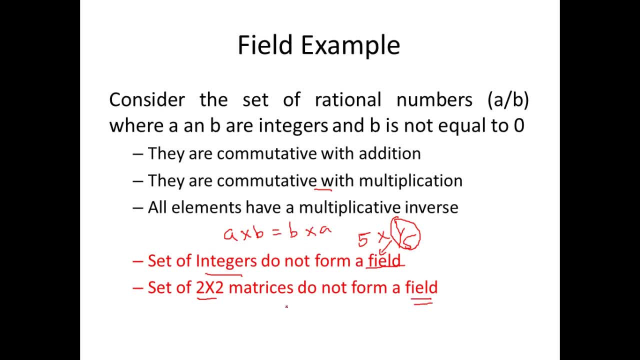 And all matrices do not have an inverse 2. So, these are some of the examples for set of elements that do not form a field. So, finally we conclude that set of all rational numbers is an example for a field and this set is actually infinite right. Set of all rational numbers is an infinite set the number of elements is infinite. 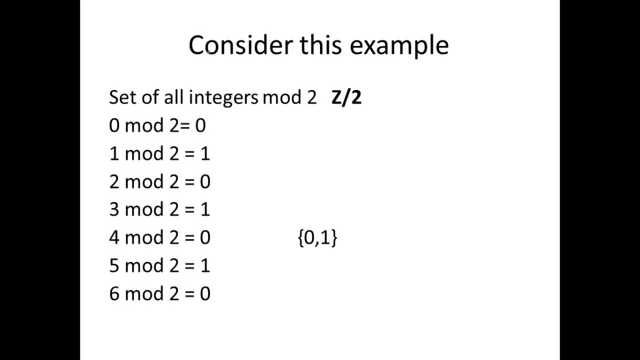 Before going into finite fields let us understand this very basic concept. This talk about set of all integers modulo 2 or else you can set of all integers mod 2. Now if you see this set of all integers 3 plus 3 is the set of all integers t plus 6 and t plus 2 is the set of all integers t minus 3 and you can see all of these numbers aretuals. So, theseU are So, what do you mean by set of all integers mod 2? It's like this your set contains all these elements say 0 mod 2 you take any element in the set we are going to do a mod 2 with that element that is the meaning of set of all integers mod 2 and it is represented like this. 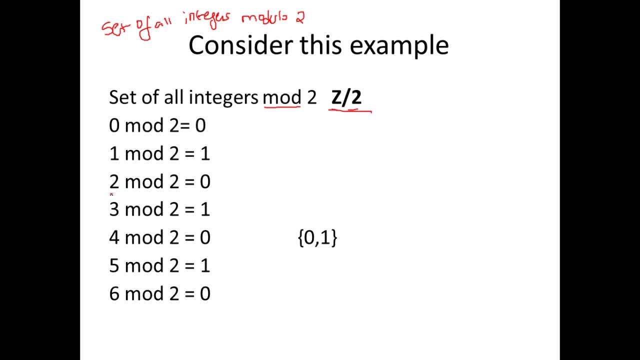 So, you take that set what will have the integer mod 2 any integer it will we have to perform a mod 2 of that integer. 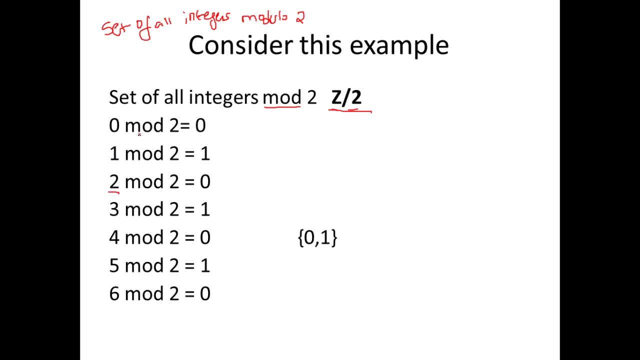 So, when you go and perform a mod 2 what will be the output say we take 0 mod 2 is 0, 1 mod 2 is 1, 2 mod 2 is 0, 3 mod 2 is 1, 4 mod 2 is 0, 5 mod 2 is 1, 6 mod 2 is 0. 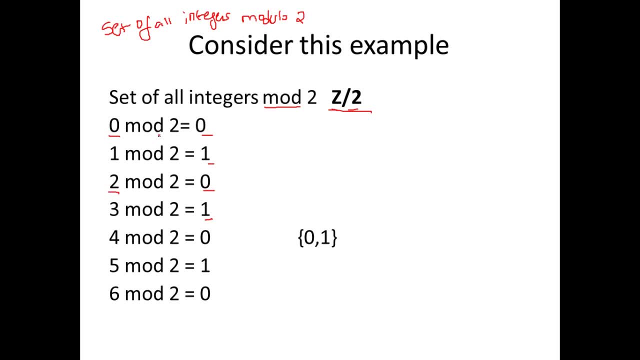 So, when you take a closer look at this when you start performing a mod 2 with the set of all integers the output is always going to be either 0 or 1. 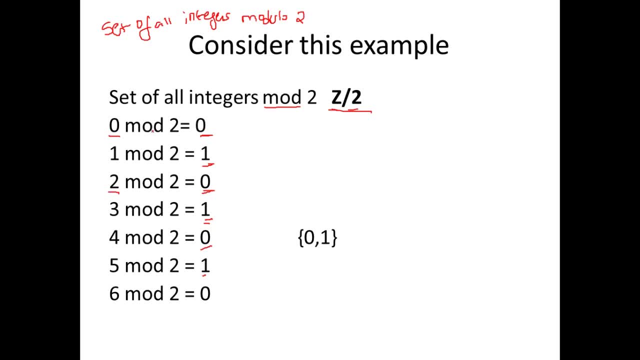 No matter how many integers you have in your set the final output is going to be 0 or 1. So, the set of all integers modulo 2 can be represented as 0 or 1. 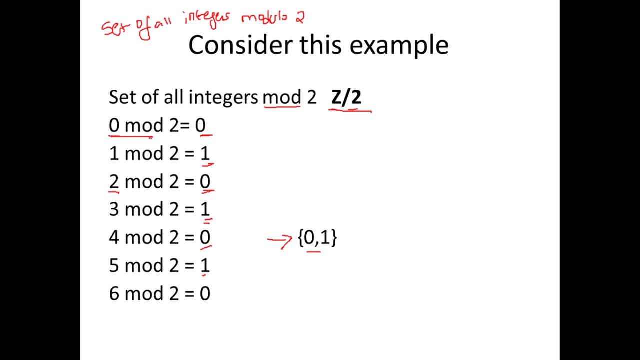 What is 0 or 1? This is nothing but representations given here. 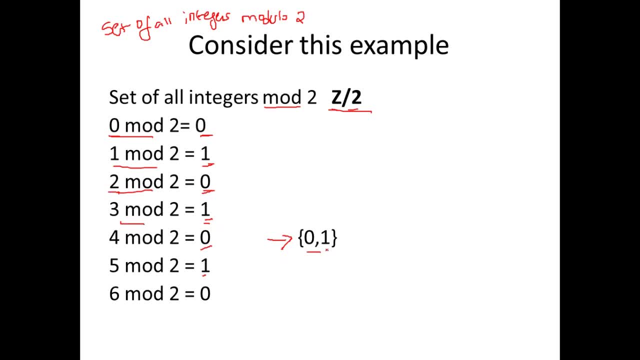 So, finally, this leads to a 0 or a 1 is that clear that is what is called the set of all integers. 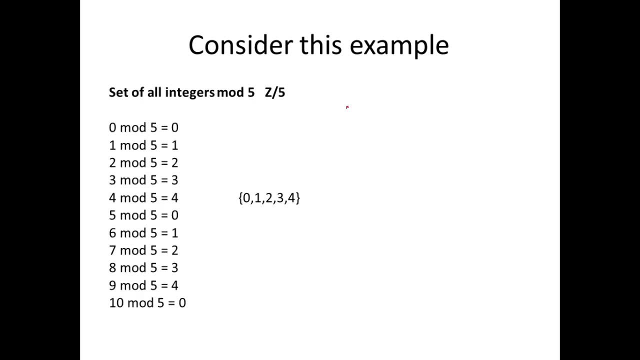 Modulo 2, likewise let us take another example set of all integers mod 5 again I have given z mod 5 here. So, what is 0 mod 5, 0, 1 mod 5 is 1, 2 mod 5 is 2, 3 mod 5 is 3, 4 mod 5 is 4, 5 mod 5 is 0, 6 mod 5 is 1, 7 mod 5 is 2, 8 mod 5 is 3, 9 mod 5 is 4 and 10 mod 5 is 0. So, again when you take a set of all integers mod 5 in this set you will have every integer wherein we take that integer and do a mod 5 and you can see a pattern here. 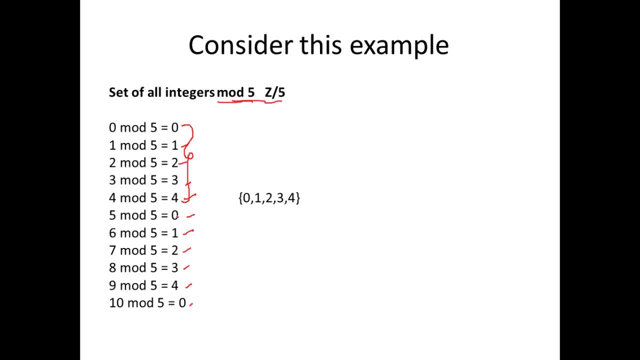 So, if the numbers the set has a value from 0 to 4 again the value starts repeating from 0 to 4. 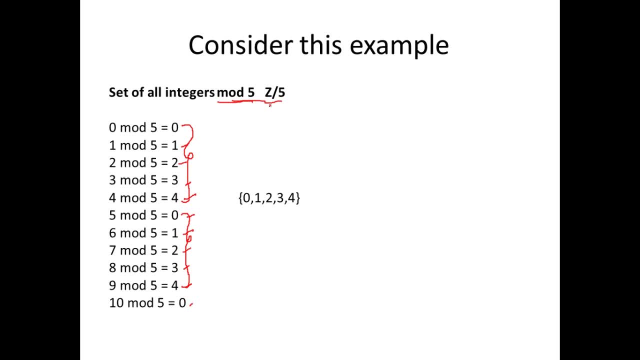 So, when you talk about the set of all integers mod 5 you are just going to have these elements. Ok. Thank you. Thank you. 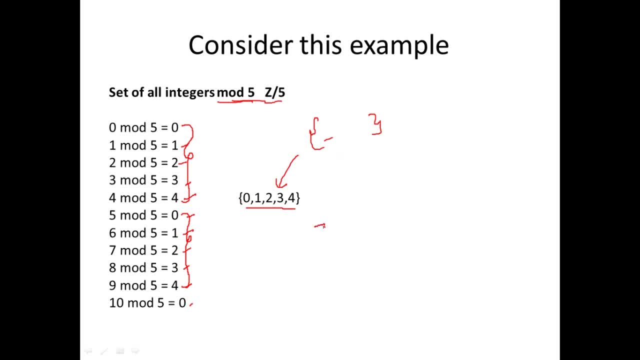 So, now we have taken two different sets that is set of all integers modulo 2 and that is represented as 0 and 1 these are the two elements in the set and set of all integers modulo 5 the elements in the set are nothing but 0, 1, 2, 3 and 4. 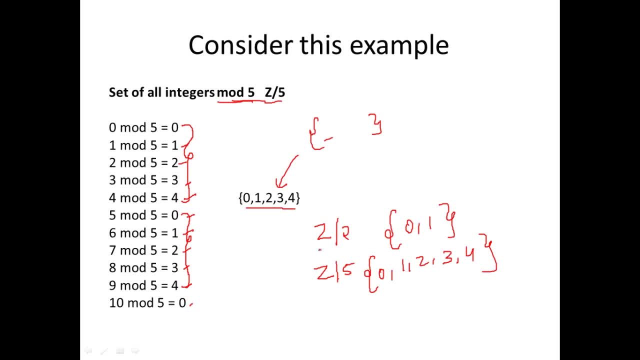 So, this is also a set now the question is, is this set a group, a ring or a field? Under what category you are going to classify these sets, that is the question. 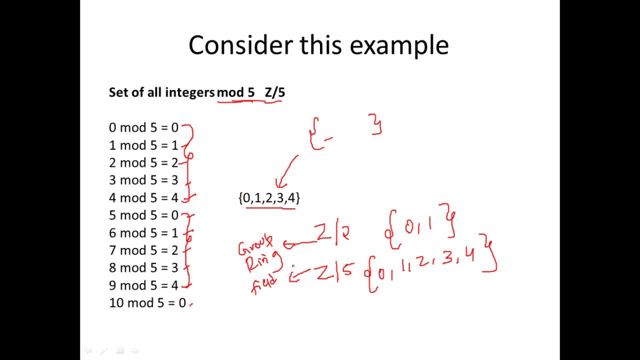 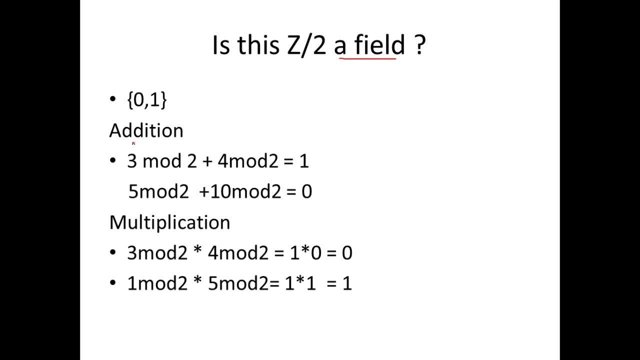 Ok, to classify something as a field what is the important property, it should satisfy addition. So, when you take addition and when you add two elements. Ok. Ok. Ok. So, you take any element in the set 3 mod 2 or 4 mod 2 when you add these two elements in the set it the result should also be part of the set. 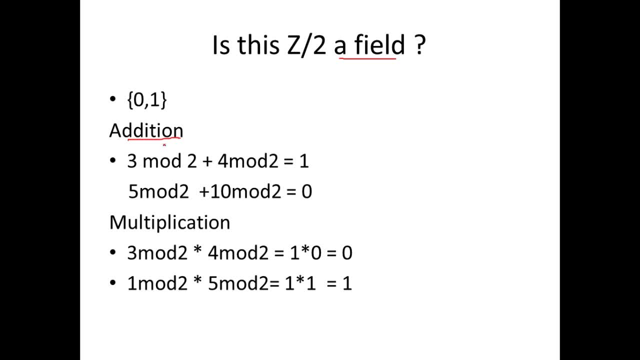 So, either 3 mod 2 it is represented as 1, 3 mod 2 is 1 plus what is 4 mod 2, 0. So, 1 plus 0 is 1, 1 is again part of the set. 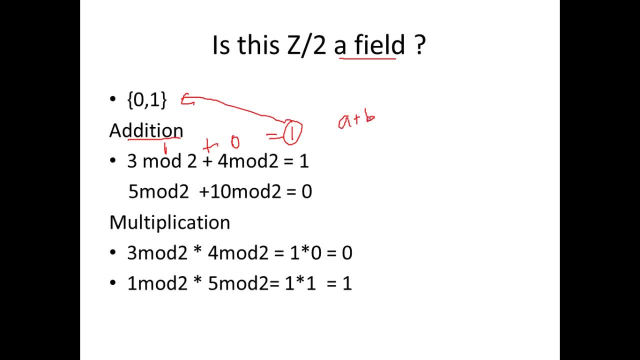 So, it is a plus b. Ok. 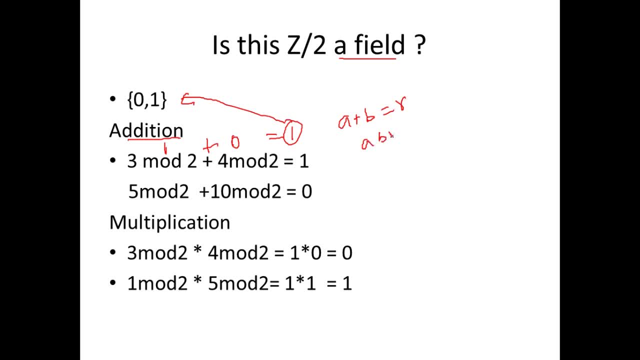 Ok. You get some result r and a, b and r belongs to g which is the set. So, that is actually called closure. 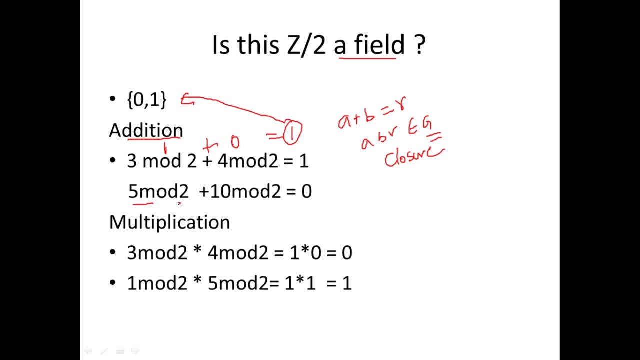 So, likewise I have taken another two elements that is 5 mod 2 which is nothing but 0 plus 0. 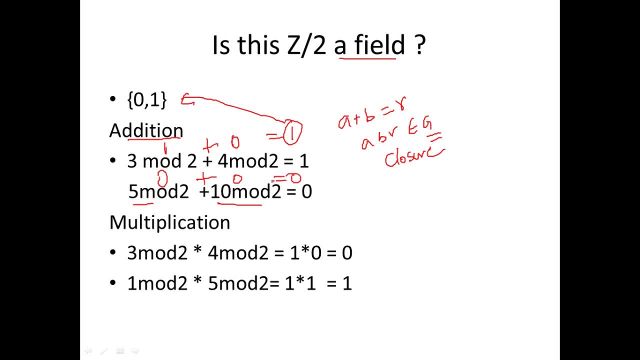 This is also equal to 0. 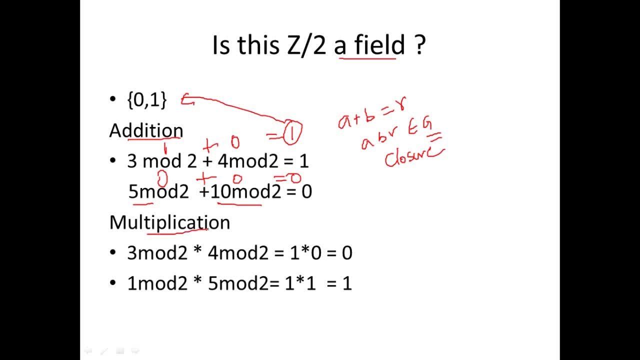 Likewise let us take multiplication 3 mod 2 star 4 mod 2 is nothing but 0. Ok. 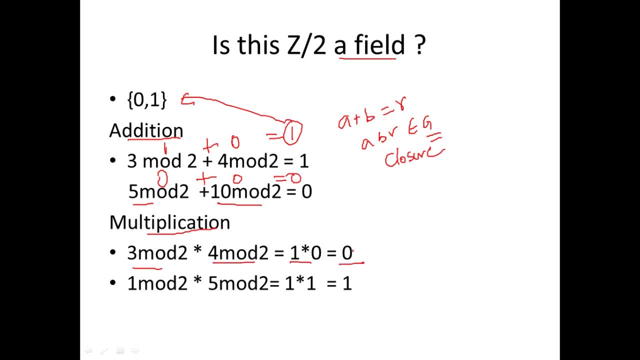 So, 1 mod 2 star 4 mod 2 is nothing but 1 star 0. The result is 0 which is again part of our set. 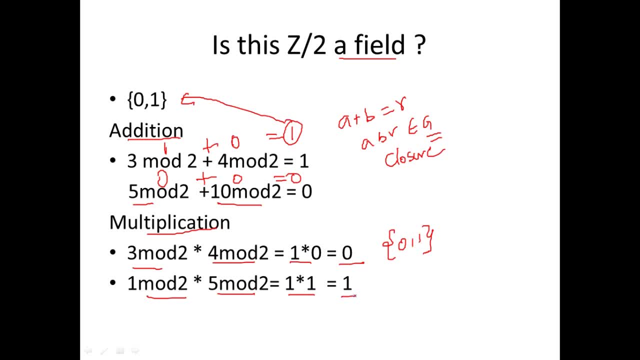 Likewise 1 mod 2 star 5 mod 2 is nothing but 1 star 1 which is again equal to 1 which is again part of our set 0 comma 1. 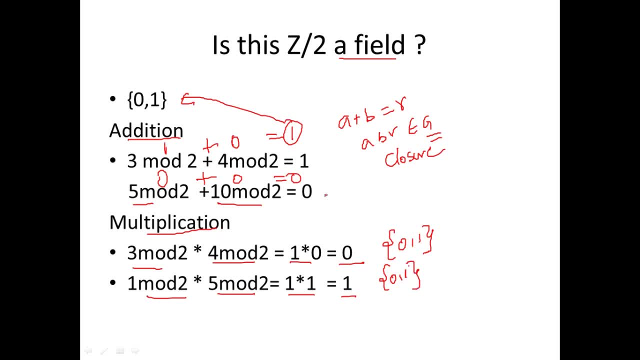 So, these operations addition multiplication are actually supported in the set of integers mod 2. 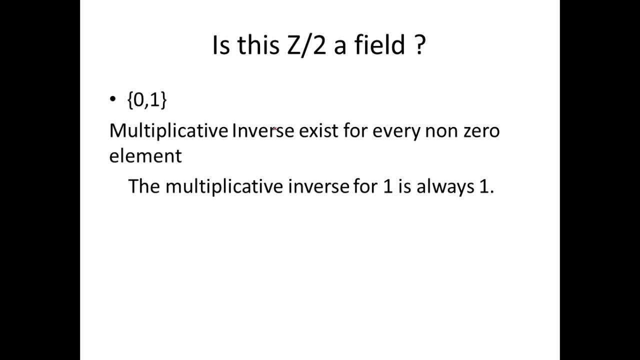 We have to check whether there is an multiplicative inverse. So, what is this multiplicative inverse? According to the definition of a field this multiplicative inverse should exist for every non-zero element. So, we are we are only worried about non-zero elements here. So, we will not worry about 0. So, the multiplicative inverse of 1 is 1. In this set for every non-zero element we have a multiplicative inverse and also addition subtraction multiplication is being supported here. 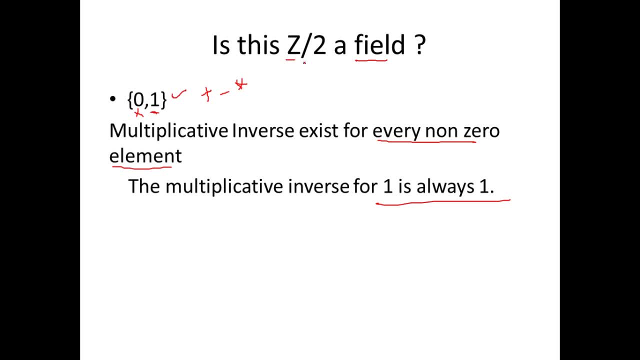 So, we can very well conclude that the set of all integers modulo 2 is a field and we go one step further. 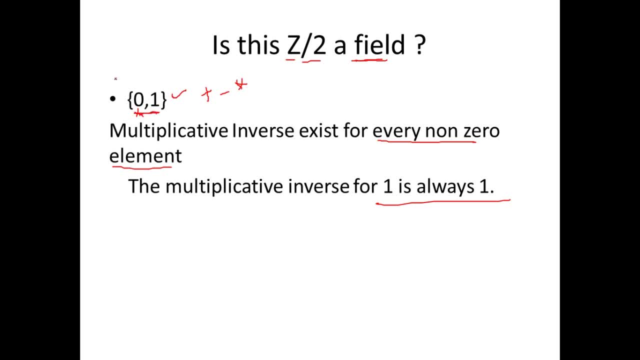 When you take this set how many fields you have here? You have only two numbers or two digits. 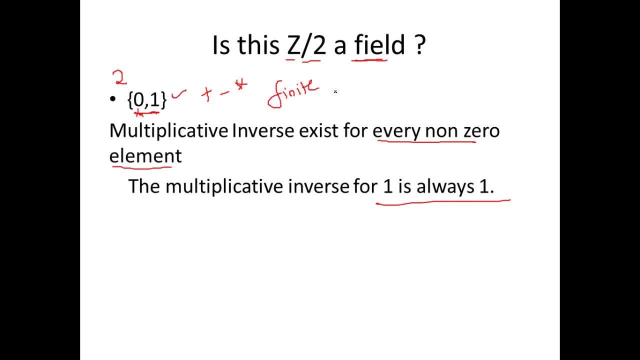 So, you have finite number of fields. That's what we understand. 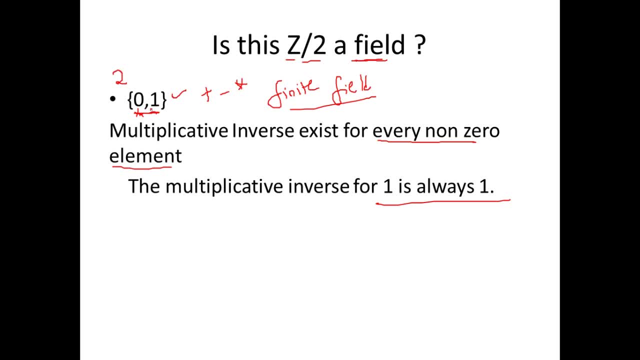 This set satisfies the properties for a field and it also contains finite number of elements. So, we can call this to be a finite field. So, that's the definition of a finite field. 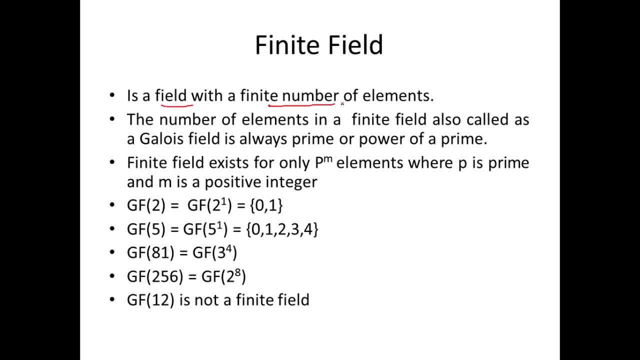 It is nothing but is a field with a finite number of elements. 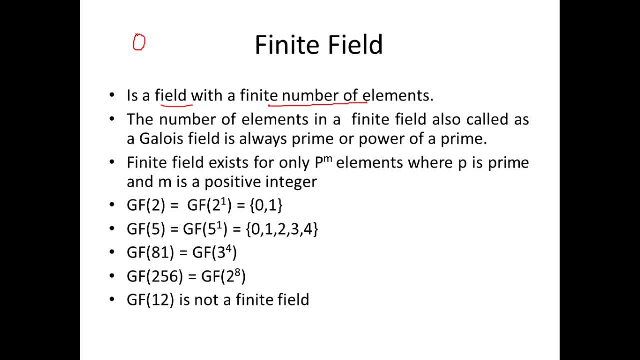 We also understood that the set of all rational numbers this is also a field right. 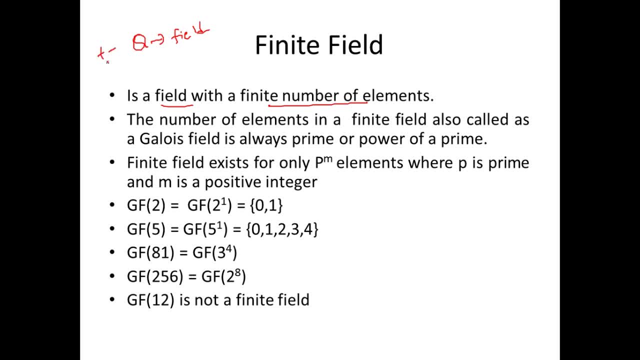 So, all the operations plus minus subtraction division was satisfied on the set of all rational numbers. 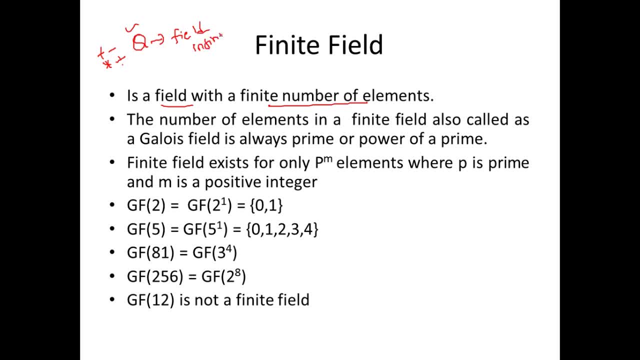 But this set add infinite number of fields whereas in cryptography we are looking for finite number of fields. We don't want infinite numbers here. 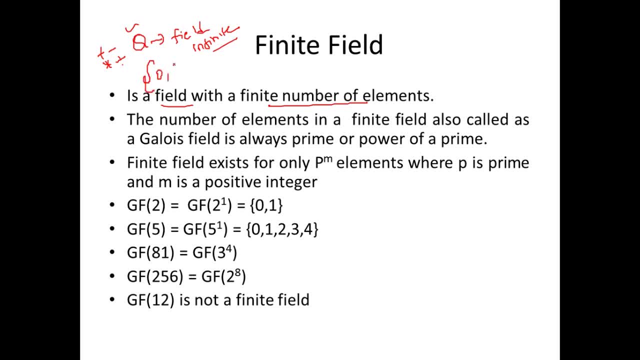 So, here when you talk about this set set of all integers mod 2 this contains finite number of fields and also it is satisfying all the properties of a field. 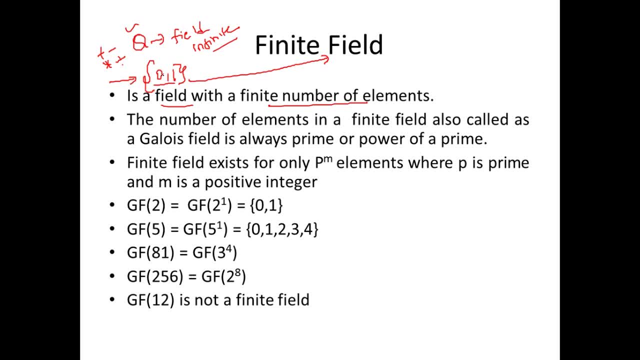 So, such sets are called finite numbers. So, there is one theory that determines how many number of elements exist in a finite field. 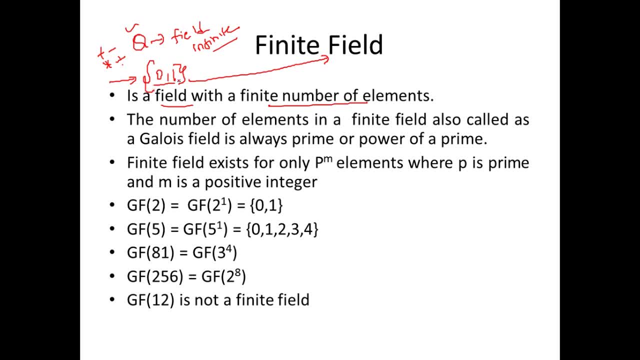 That's the theory that says how many number of elements will exist in any finite field. 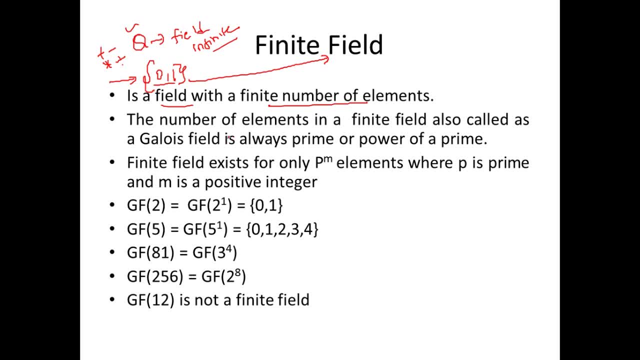 So, that is this theory that is number of elements in a finite field. 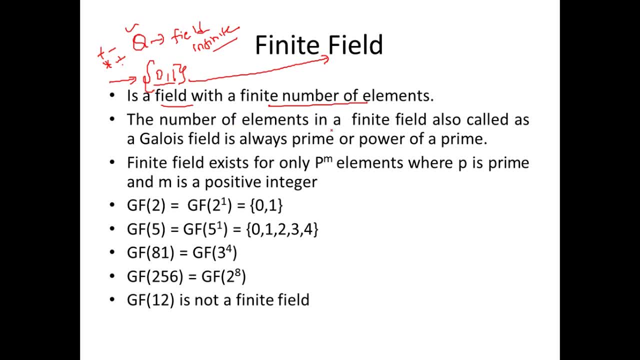 This finite field is also called as a Galois field based on the person who discovered this. So, this is the theory that is number of elements in a finite field. 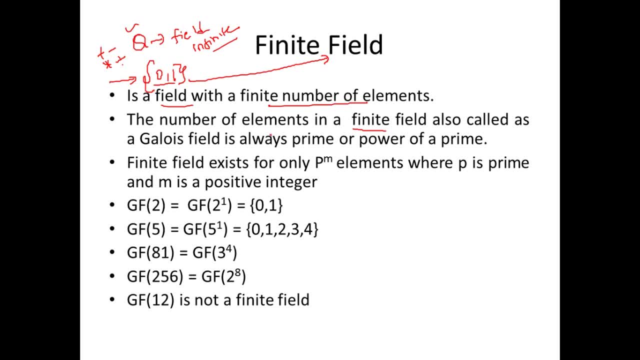 And the number of elements in a finite field is always prime or power of a prime. A finite field exists only for p per m elements where p is a prime number and m is any positive integer. 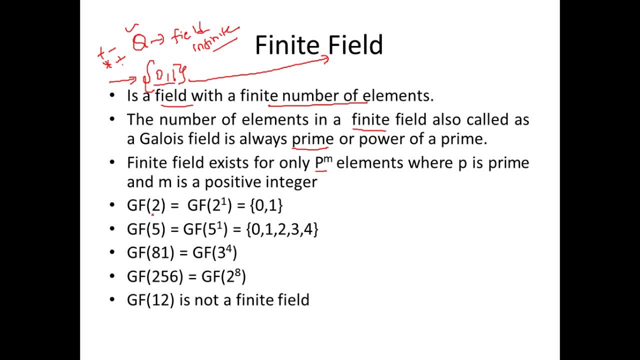 Let's take some example. We have already taken 2. 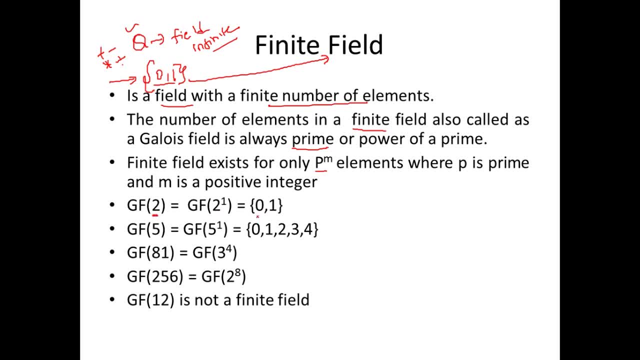 What is this set of 2? It is nothing but 0 and 1. And 2 is 0. And 2 is a prime number. 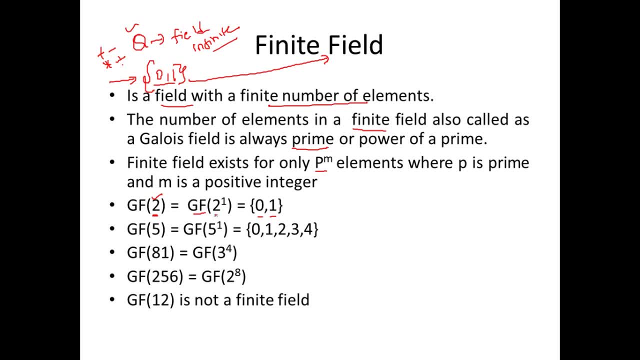 We can also represent this as Gf 2 per 1 where Gf is nothing but a finite field or a Galois field. 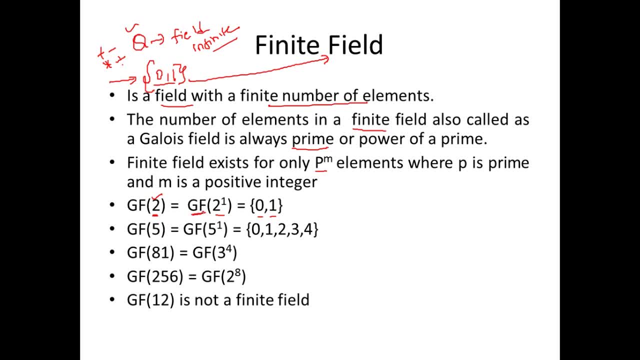 So, what is this Gf? Gf is a Galois field and it represents a finite field containing 2 elements 0 and 1. 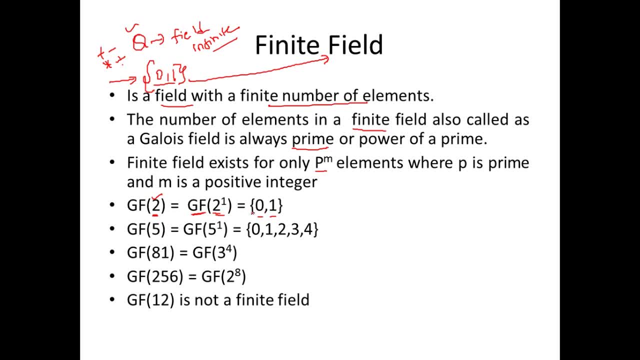 For a set to be a finite field, the very important property is this number should be a prime number. 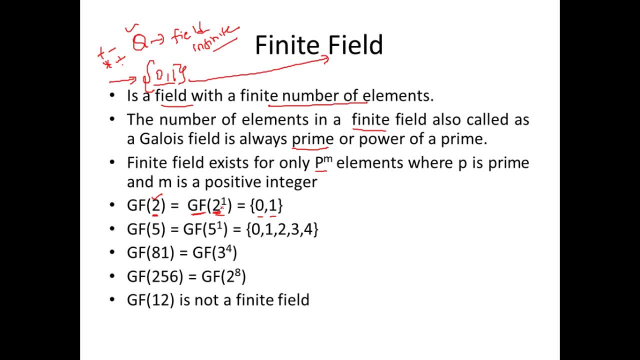 This number should be a prime number and it can be raised to power of any positive integer. 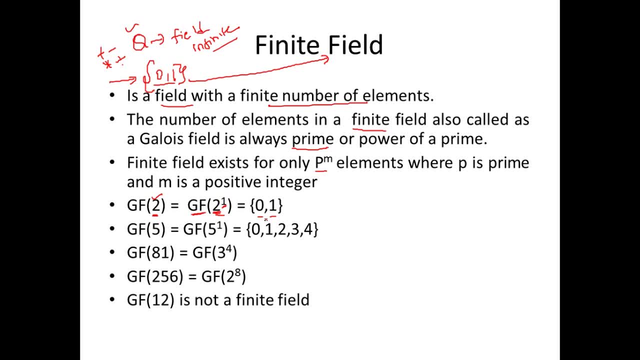 Here, Gf of 2 is nothing but 2 per 1 is nothing but Gf of 2 that is this. 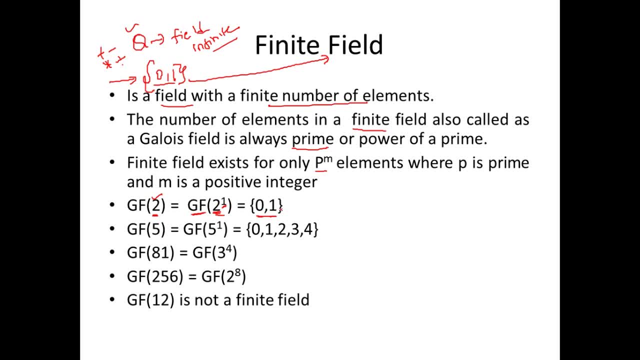 Likewise, 5 is also a prime number. So, it also creates a set of finite fields or Galois fields. 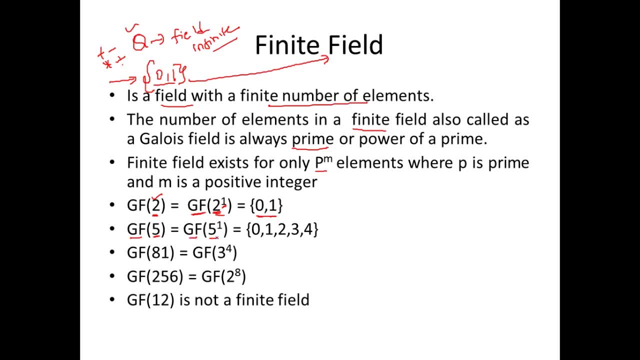 And we can also represent this as Gf 5 to the power 1. 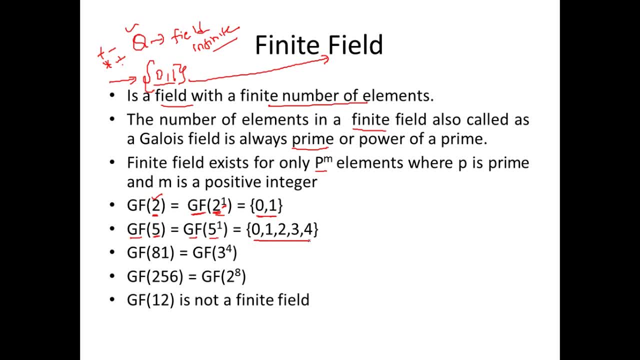 So, how many elements you add in this set? 0, 1, 2, 3, 4. 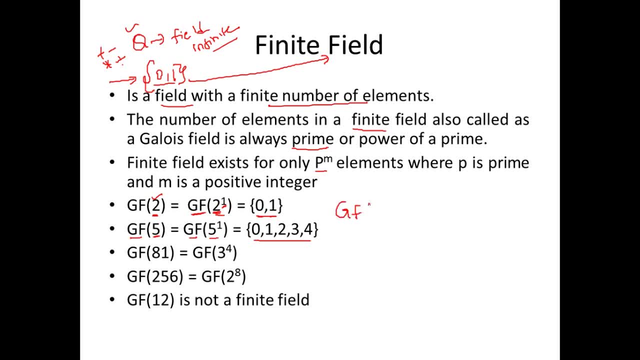 For any finite field, if the element is a prime number, say if this is prime, then how many elements you will have in the set is nothing but 0 to 7 minus 1. 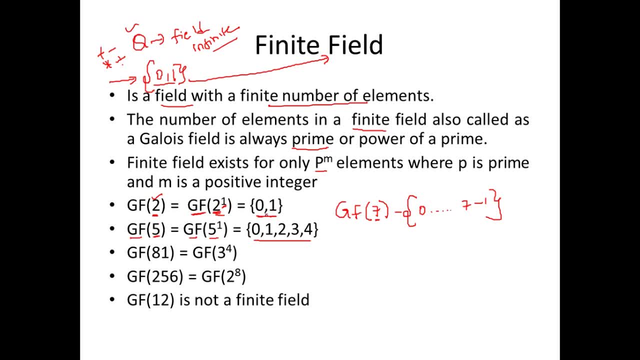 We know 0, 1 is a finite field and it can be represented as Gf of 2. And how many elements you have? 0 to 2 minus 1. Likewise, for Gf of 5, how many elements you have? 0 to 5 minus 1. 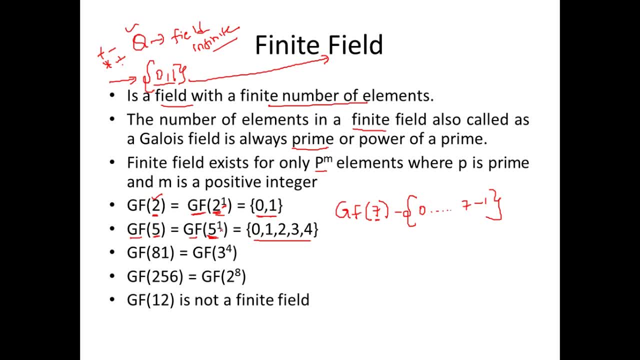 The only criteria is this number should be a prime raised to the power of any positive integer. So, finite field 81 and this can also be represented as 3 to the power 4. So, there is a finite field 256 elements and this is represented as 2 per 8. So, this we will be using that in advanced encryption standard. 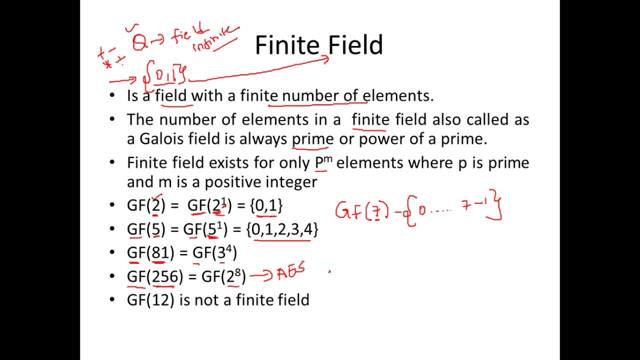 So, what is this 2 per 8? It is nothing but you can just think that to be 8 bits, right? 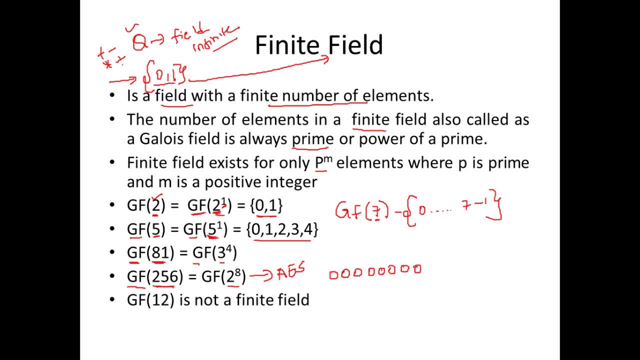 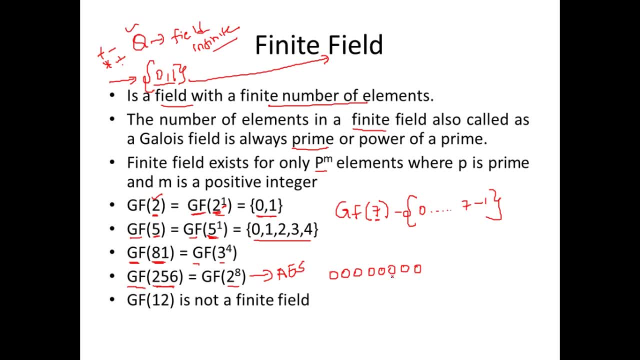 So, we have 8 bits here. 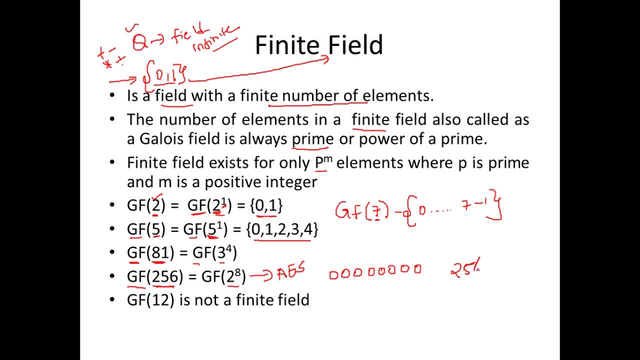 And what is 2 per 8? So, we will have 256 different values. 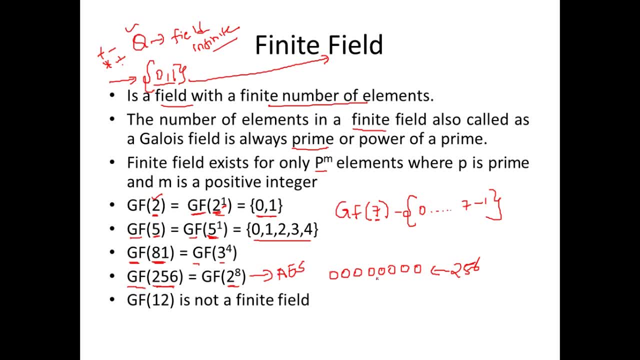 And since it is G of 2, what are the possible values here? Either it can be 0 or 1. 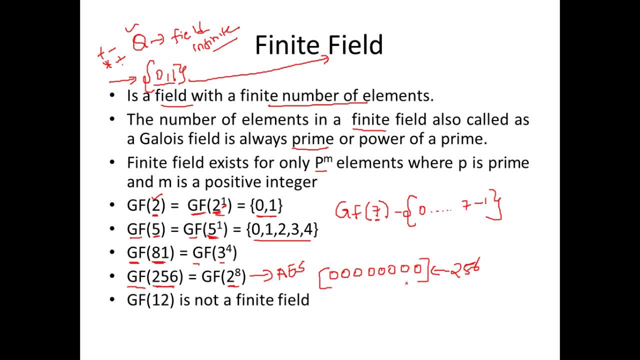 And since it is a finite field, what do you mean by a finite field? All these operations plus, minus, division, multiplication can be performed on these 256 elements. 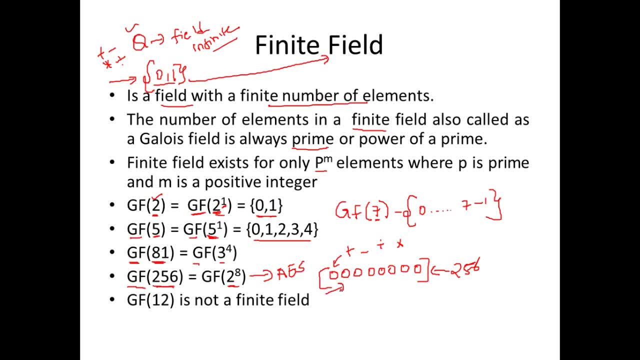 The result will also be part of this set. 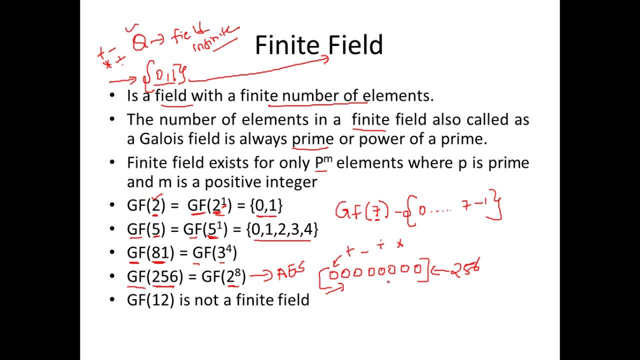 So, it is nothing but 256 different byte combinations. That's it. 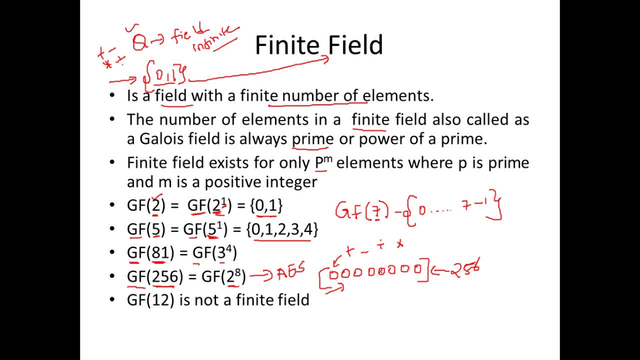 That forms a set and you call that to be a finite field because all these operations when you perform on that set, you are going to get a result which is also part of the set. 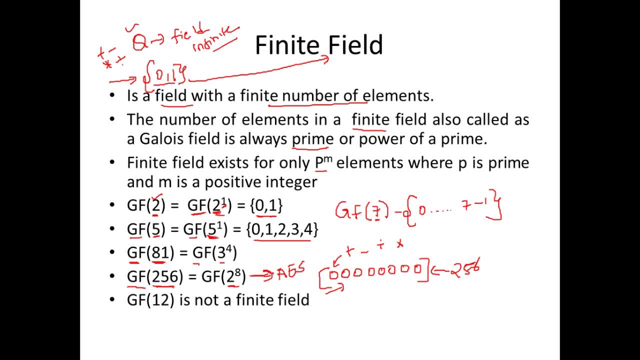 And in advanced encryption standard, we will be focusing on finite fields that is represented as G of 2 per 8. 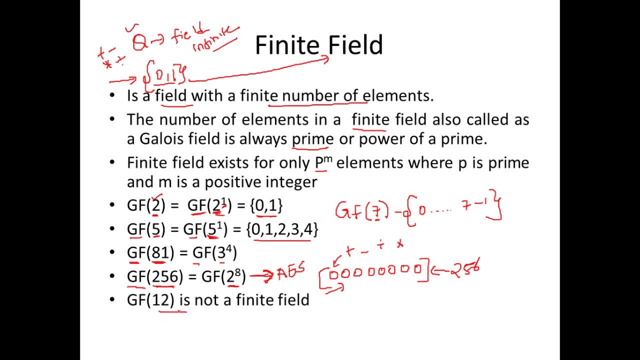 Is G of 12 a finite field? It is not a finite field because you can't represent 12 as a finite field. It is a power of a prime. 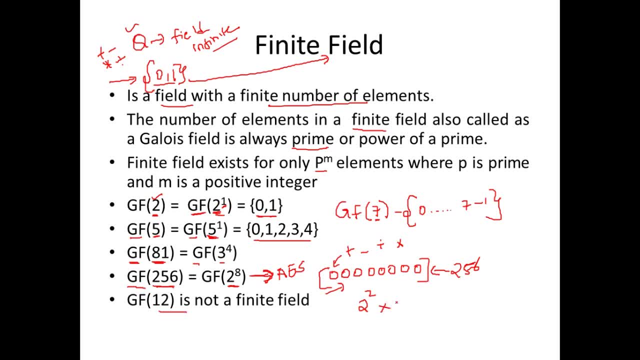 You can say 2 square star 3, but this is not of the form p power m. So, we can say that G of 12 will not form a finite field, will not form a set of finite field elements. 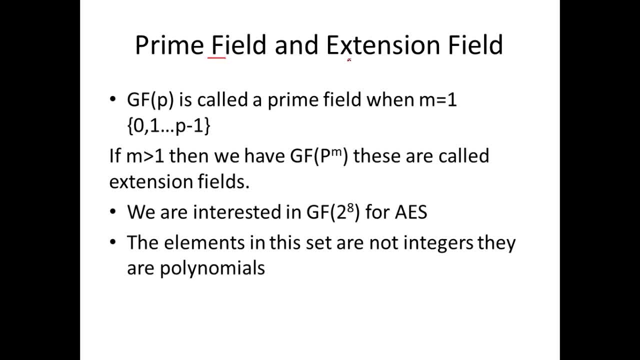 Now we have to look at the difference between prime field and extension field. It's very simple. Say in Galois field of P if M is equal to 1 we say that is a prime field 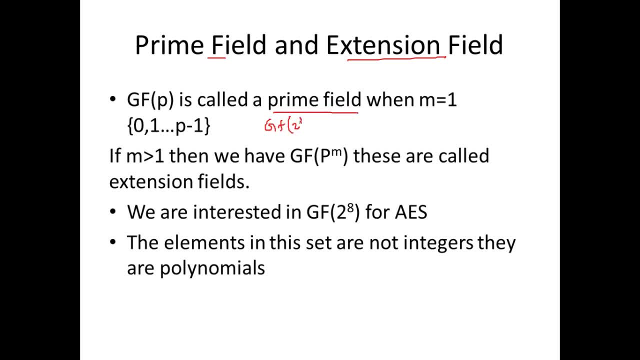 So GF of 2 power 1 so here M is 1 so we say GF of 2 to be a prime field 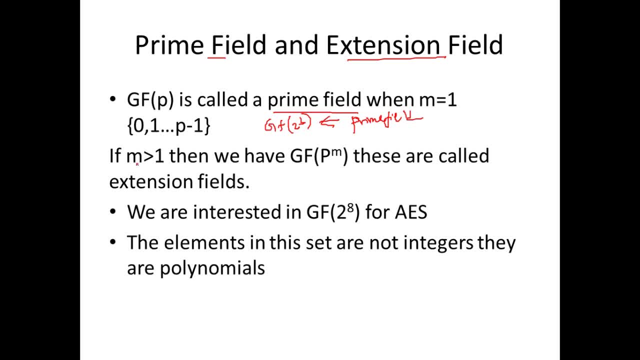 If M is greater than 1 then we say such fields are called as extension fields I have showed you GF of 2 power 8 this is what we are interested in AES right 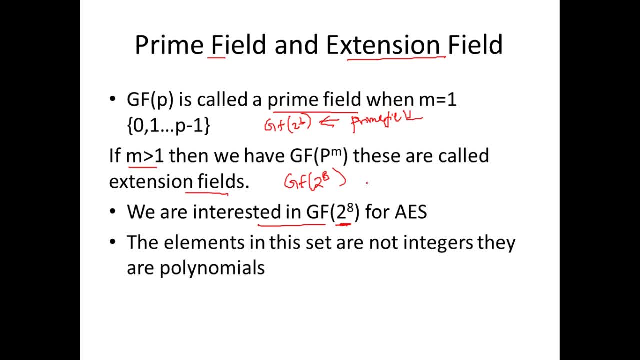 So 2 power 8 when we have M to be greater than 1 we call that to be an extension field Another thing that we have to understand here is we know that a set of integers will contain all integers 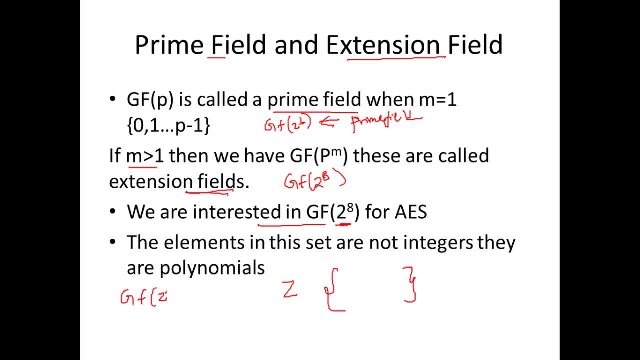 Whereas a set of finite fields with P is equal to 2 We know that a set of finite fields with P is equal to 2 will contain all integers Whereas a set of finite fields with P is equal to 2 will contain all integers Will contain two elements 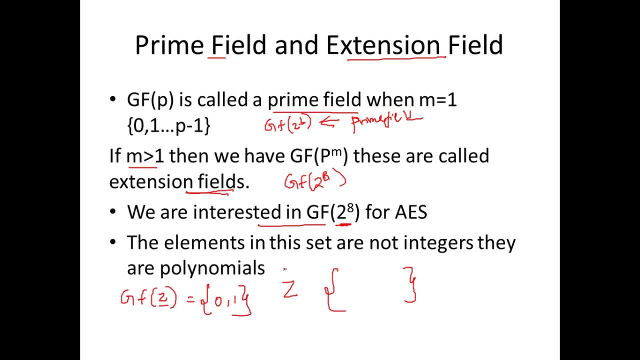 Whereas when you talk about a finite field a set 2 power 8 it is made up of polynomials It may be shocking to you but that is what it is 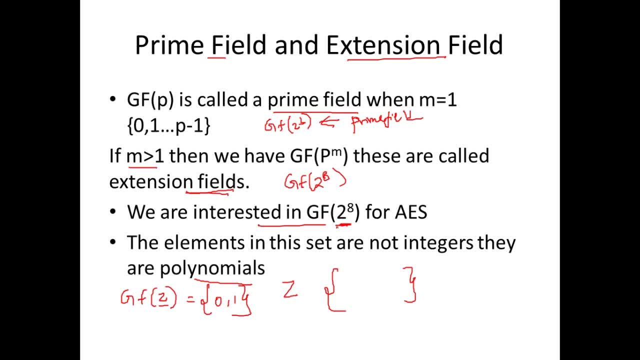 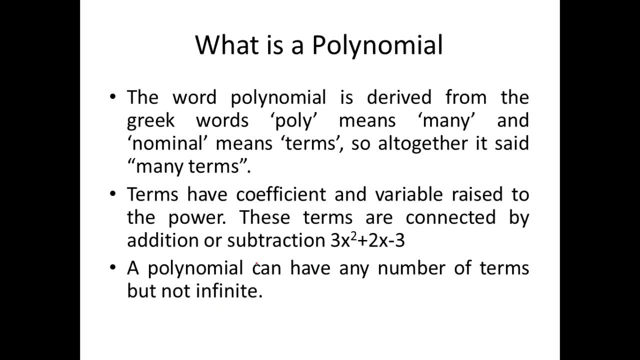 The elements in this set they are not integers they are polynomials So I hope you all know what is a polynomial right Polynomial is nothing but many terms attached together using the addition or subtraction operation And in a polynomial you will have a coefficient and a variable And these terms so a coefficient plus a variable together makes a term Like that many terms will be attached together using a subtraction or an addition or a subtraction So that becomes a polynomial In polynomial you can have many number of terms but the number of terms will not be infinite So this set Corresponding to g of 2 power 8 that is nothing but a set of all polynomials We are talking about this finite field right This finite field will be having set of polynomials So when I say 2 power 8 every polynomial will have 8 terms So it can be plus plus plus plus plus like that 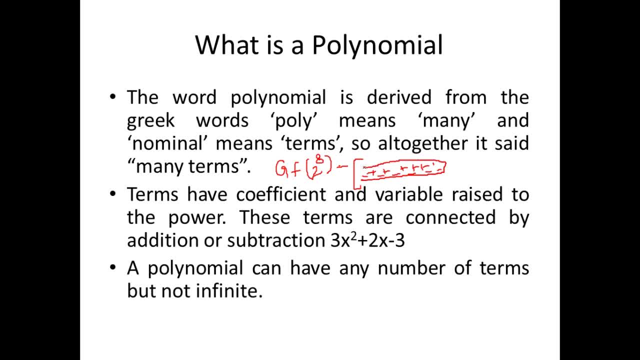 So it can be plus plus plus plus like that So a polynomial of 8 terms will make an element in this set 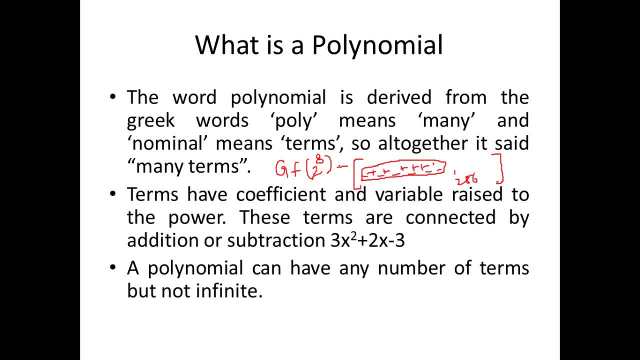 Likewise I will have 256 different elements So we are going to work with polynomials in our advanced encryption standard 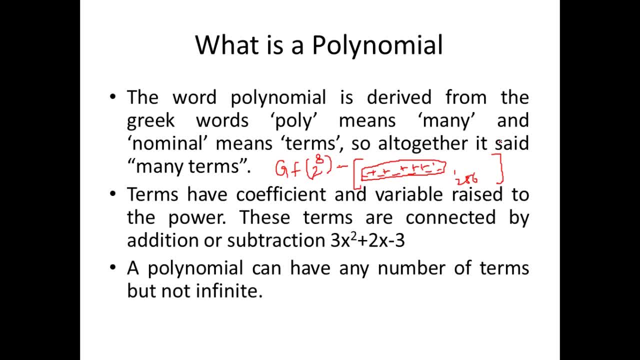 So that forms the basics and we will be again revisiting this later on 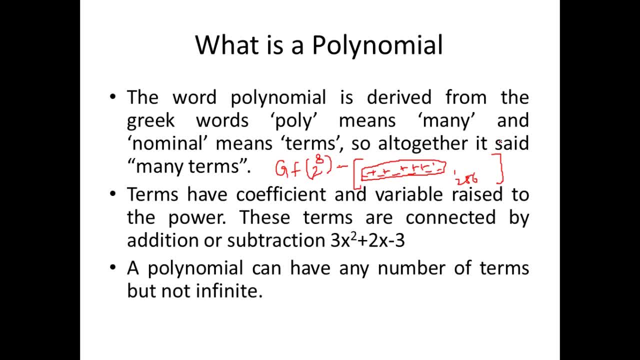 I hope you all have understood what is a group What is a ring What is a field The properties of groups, rings and fields 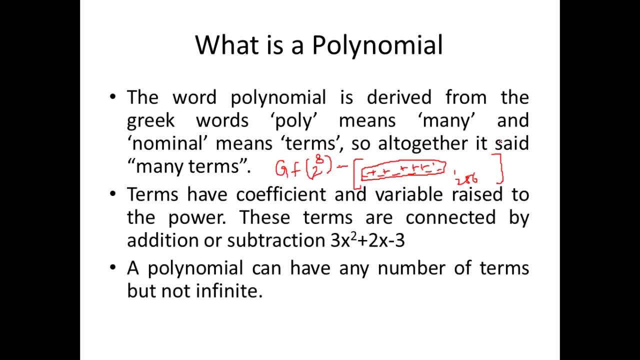 And what is integer modulo 2 The set of all integers modulo 2 And the set of all integers modulo 5 And we have seen how these two sets satisfy the properties for a field 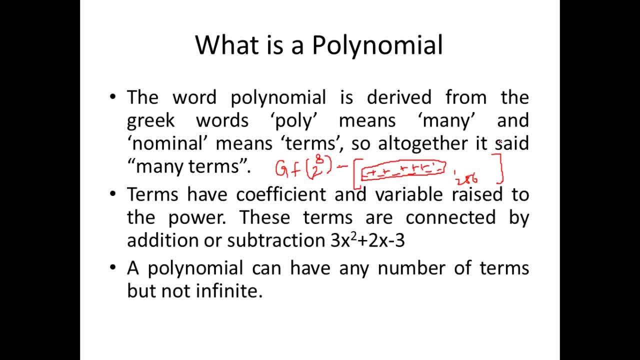 And why we say these are finite fields Because they have a finite number of elements 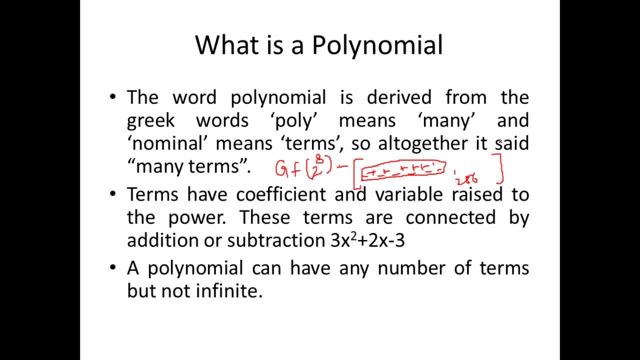 And they satisfy the properties for a field And then we looked at What is more important for us to understand For advanced encryption standard 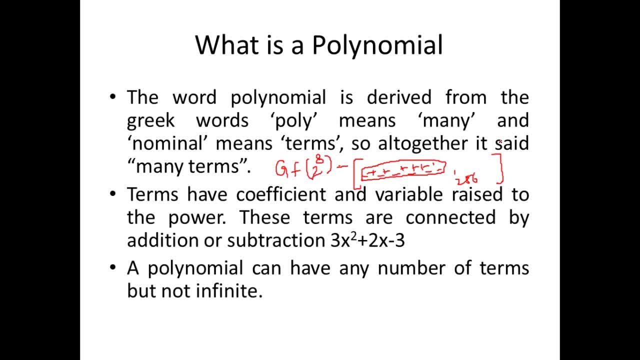 It is the finite field represented in the format 2 power 8 It just means we are going to have a polynomial with 8 terms for every element And there will be 256 different polynomials like that And when we apply the concepts of addition, subtraction, multiplication or division on these polynomials We are going to get the result to be again part of the set And it will also be a polynomial 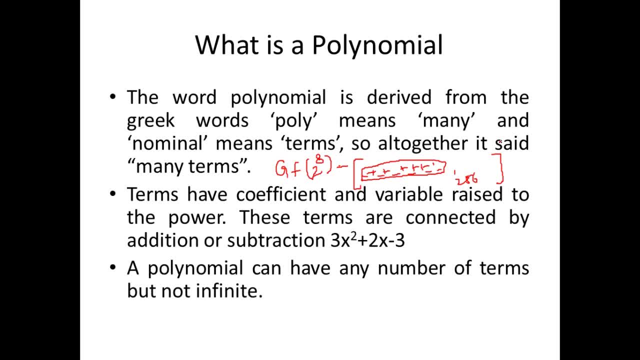 So this concept we will be using that in Advanced encryption standard Thank you 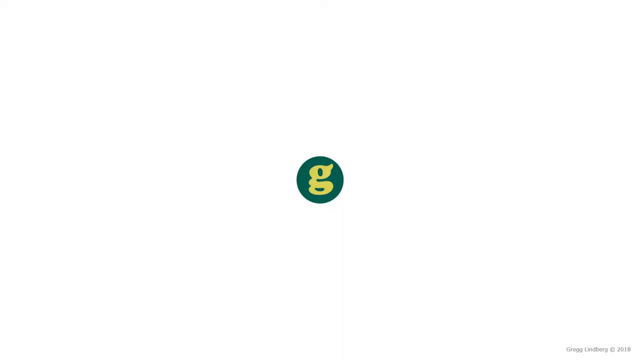 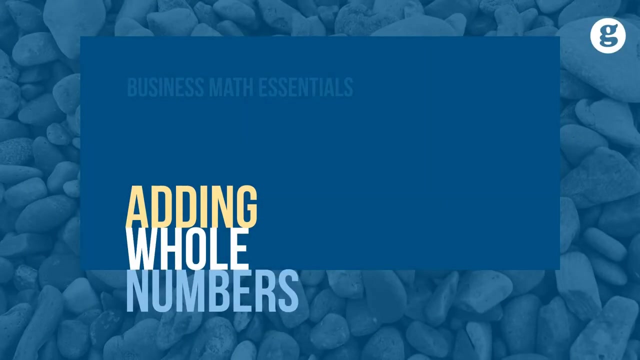 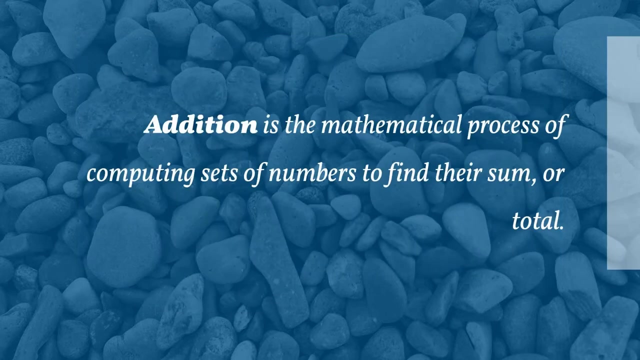 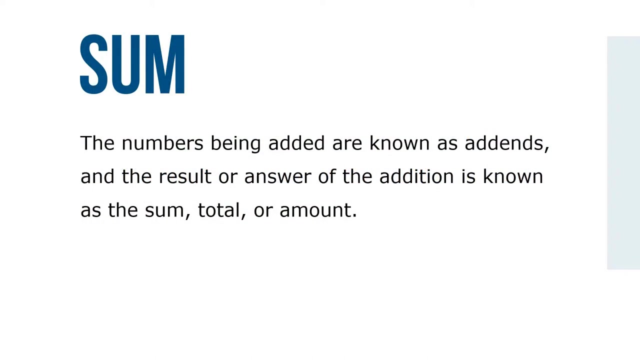 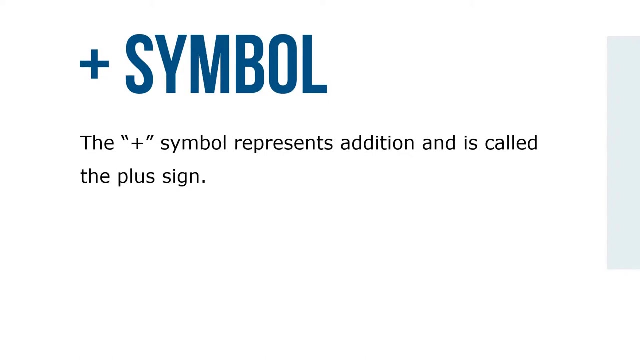 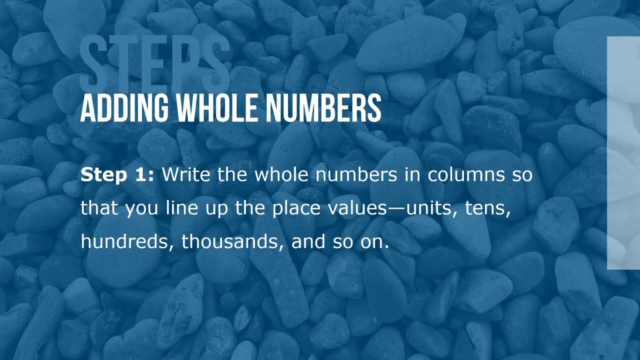 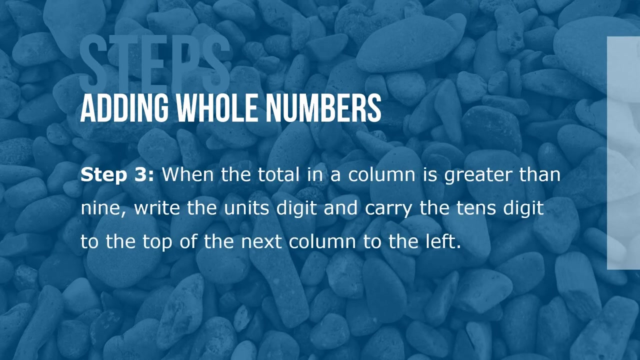 Addition and subtraction are the most basic mathematical operations. They're used in almost all business calculations. In business, amounts of things or dollars are often combined or added to determine the total. Let's take a look at adding whole numbers. Addition is the mathematical process of computing sets of numbers to find their sum or total. The numbers being added are known as addends, and the result or answer of addition is known as the sum, total, or amount. The plus symbol represents addition and is called the plus sign. Here are the steps for adding whole numbers. Step 1. Write the whole numbers in columns so that you line up the place values. Units, tens, hundreds, thousands, and so on. Step 2. Add the digits in each column, starting on the right with the units column. Step 3. When the total in a column is greater than 9, write the units digits and carry the tens digit to the top of the next column to the left. 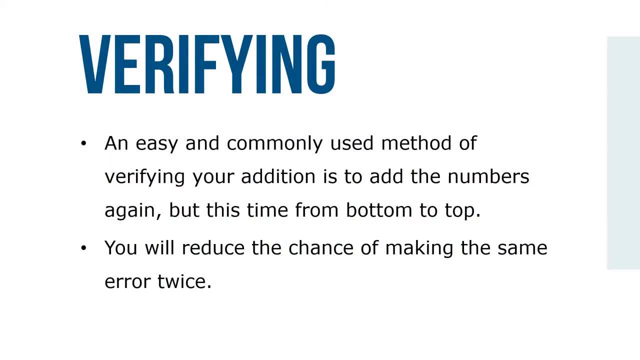 Generally, when adding the digits in each column, we add from top to bottom. An easy and commonly used method of verifying your addition is to add the numbers again, but this time from bottom to top. By adding the digits in reverse order, you'll reduce the chance of making the same mistake twice.